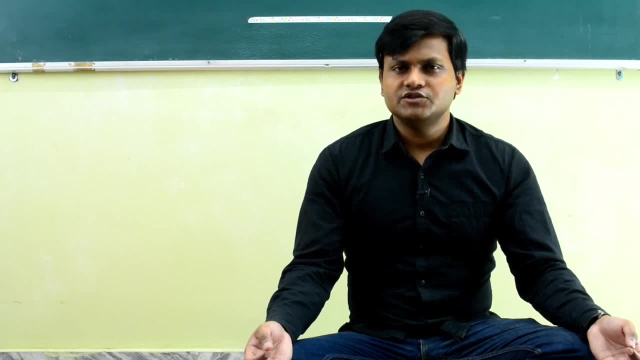 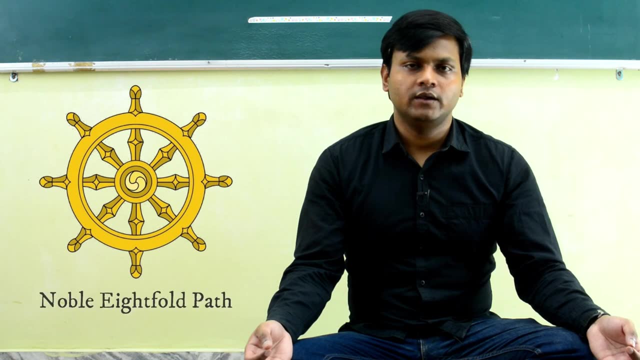 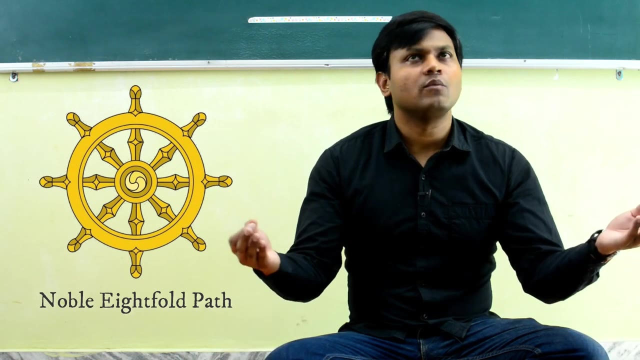 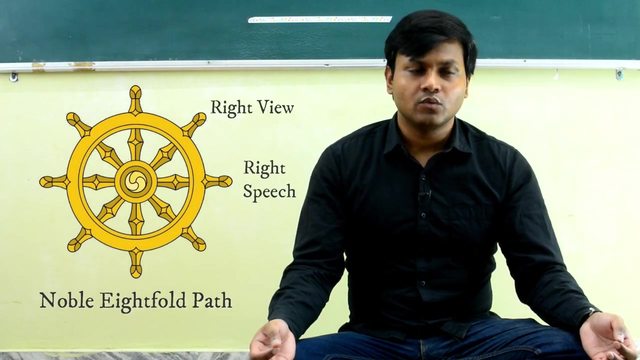 In the ancient philosophy of Buddhism, there is what is called the Noble Eightfold Pathway, which simply consists of eight practices that can lead to enlightenment or freedom from samsara. They consist of the right view, the right speech weight. This was supposed to be a video on 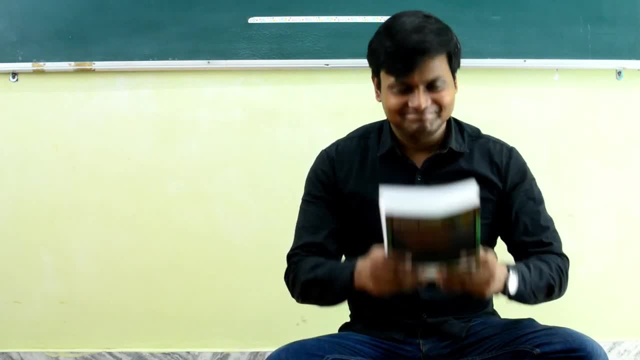 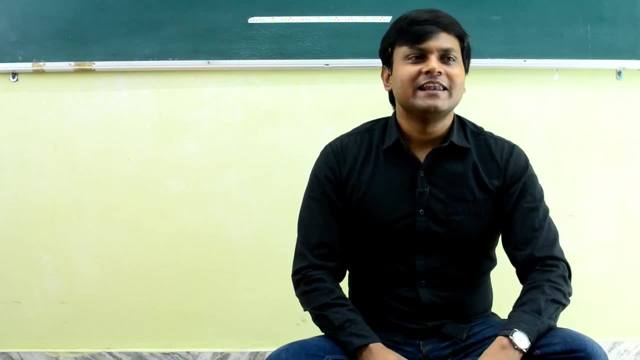 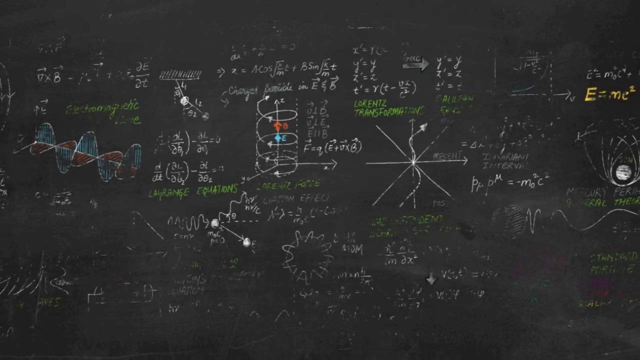 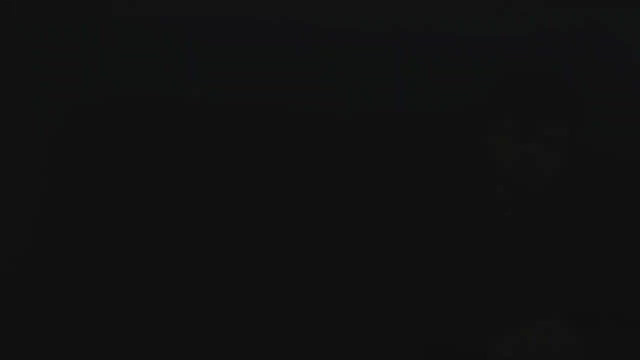 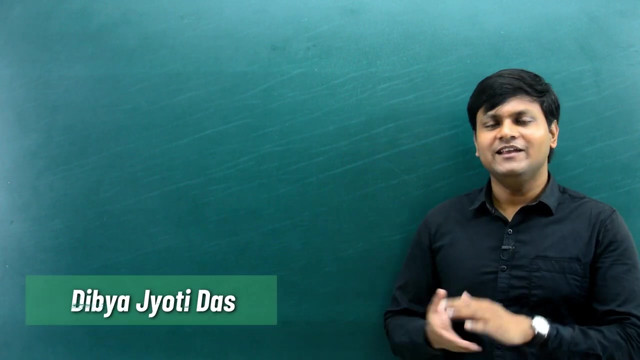 particle physics, right. Okay, I got confused again. I'll talk about this in some other video. Let's do the video of particle physics, Okay. so the Eightfold Way in particle physics, as opposed to the Eightfold Path in Buddhism, is a classification of subatomic particles. Now. 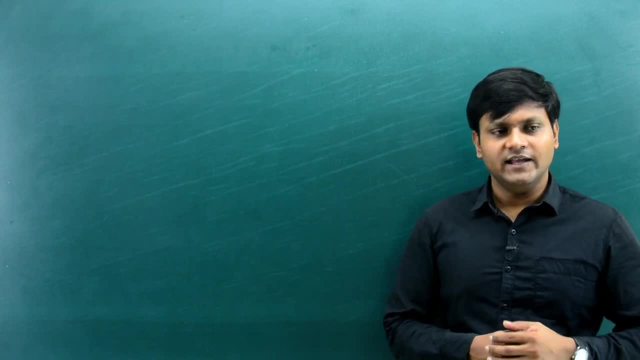 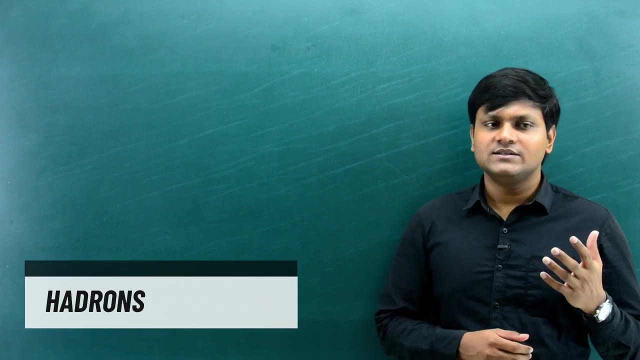 if you have followed my earlier videos on particle physics, then in one of my earlier videos I have talked about the class of particles called hadrons. So hadrons are a class of particles that experience the strong force And, as it turns out, there are a large number. 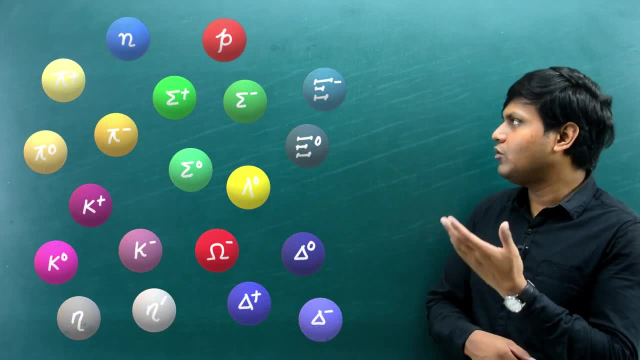 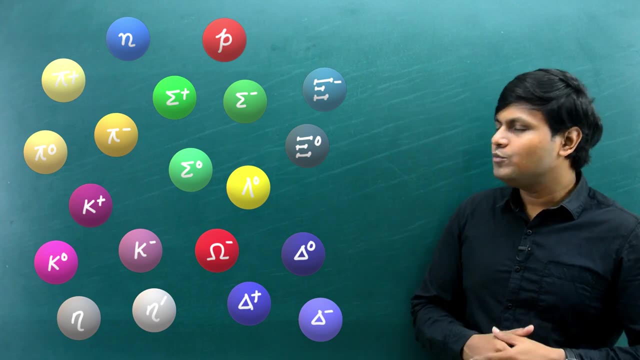 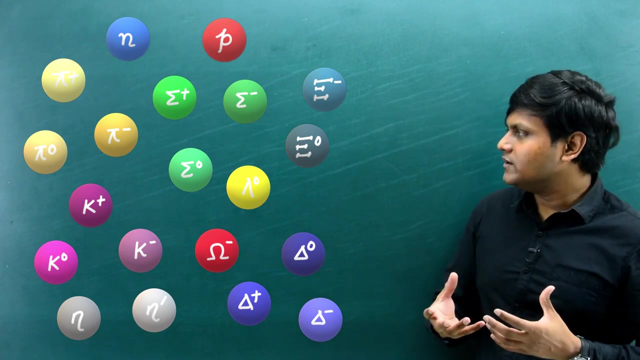 of hadron particles out there. You have the usual neutron proton, you have the pie meson, these sigma particles, these i particles, omega particles, kaon particles and on and on and on. One very simple question that you may ask is that: are these particles fundamental? Are these? 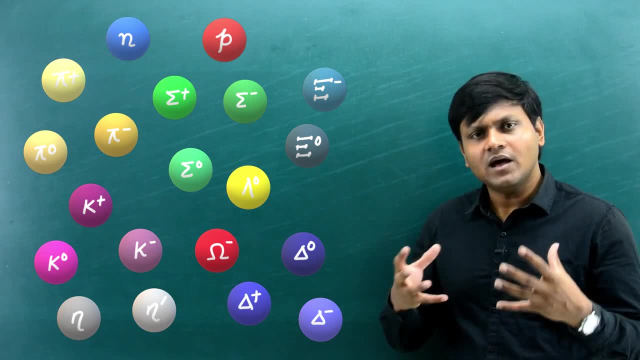 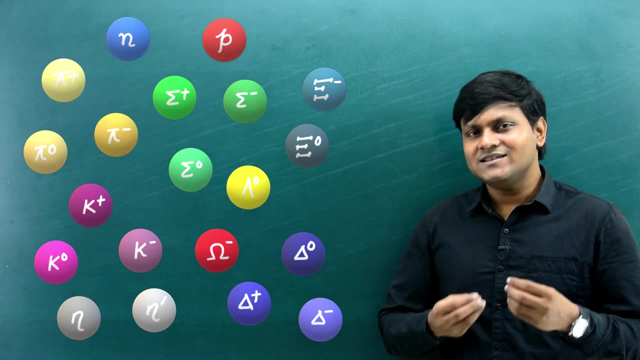 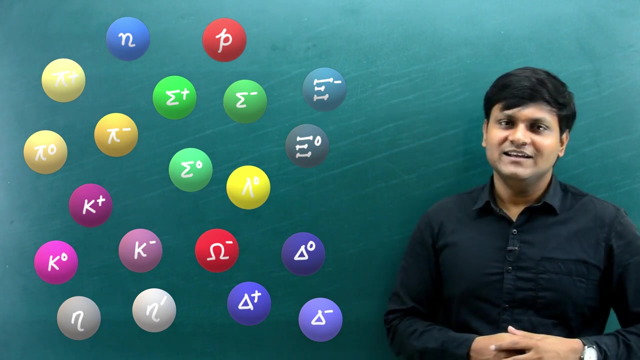 particles elementary, That is, are they made up of more elementary particles or are they elementary on their own? And to answer that question we need to look at this Eightfold Way in particle physics. So one of the earliest ideas of combining these kind of particles into 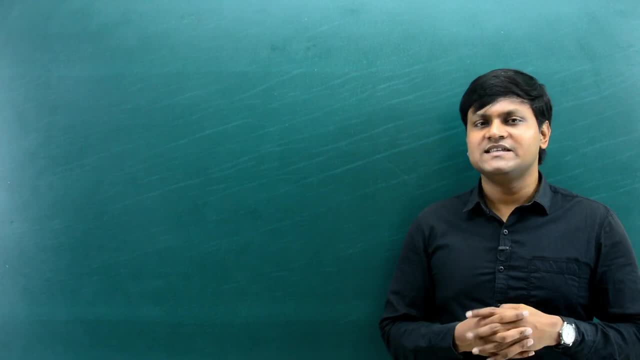 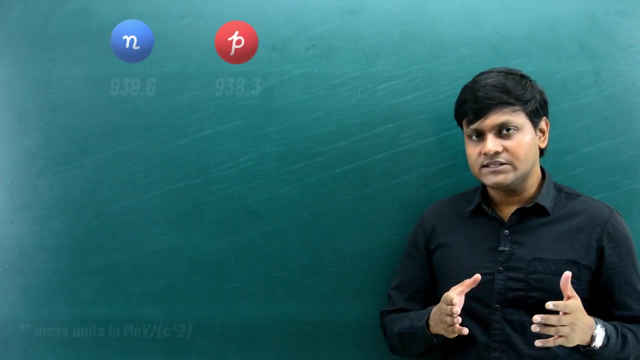 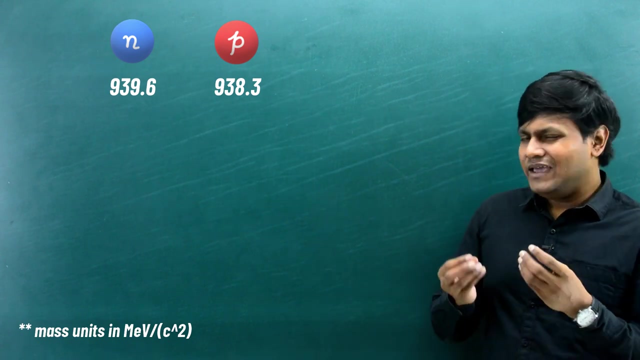 fundamental entities consisted of organizing particles into multiplets. So, for example, if you look at the neutron and the proton, they seem to have similar mass but different charge. Neutron is neutral, proton is positively charged, So it was thought that maybe, maybe they are the 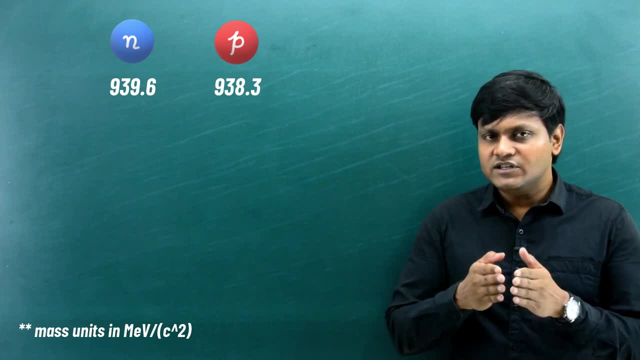 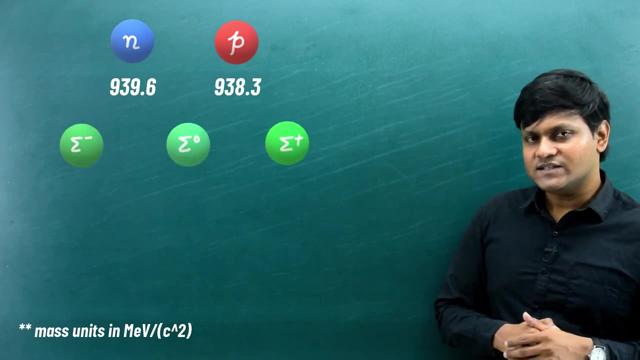 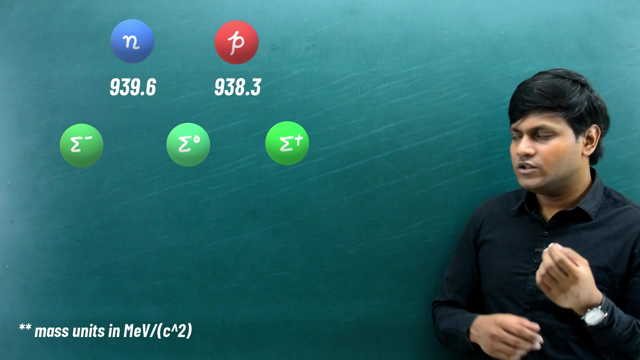 result of a fundamental entity But having different charge states. You can see other groups also. For example, if you look at the sigma group, if you look at the sigma particles- sigma plus, sigma zero and sigma minus- the superscript simply represents the charge. The plus, zero and minus represents plus one electronic. 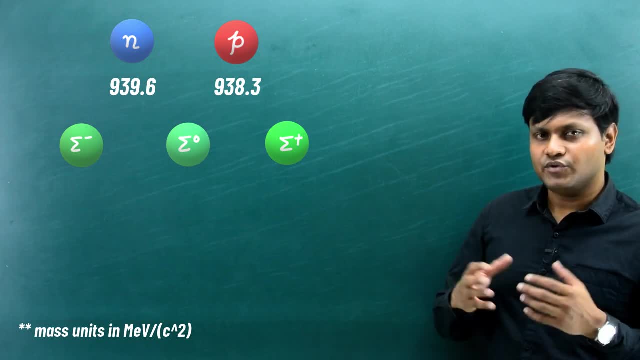 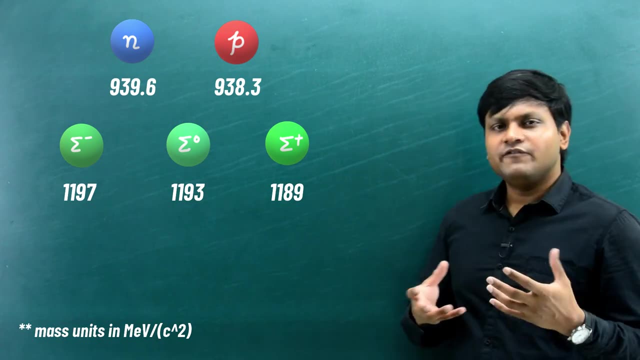 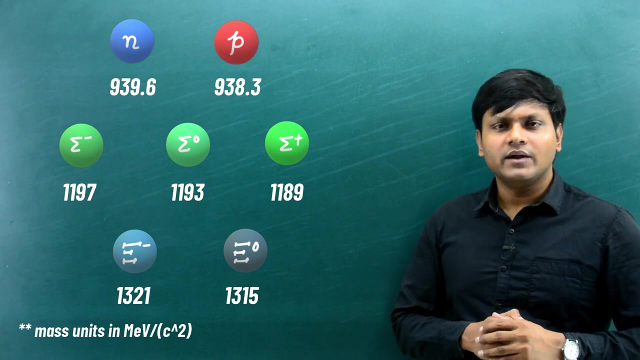 charge, zero electronic charge and minus one electronic charge respectively. They also have similar masses And it was thought that even maybe they are the result of a fundamental entity having different charge states as well as these xi particles. So these are groups of 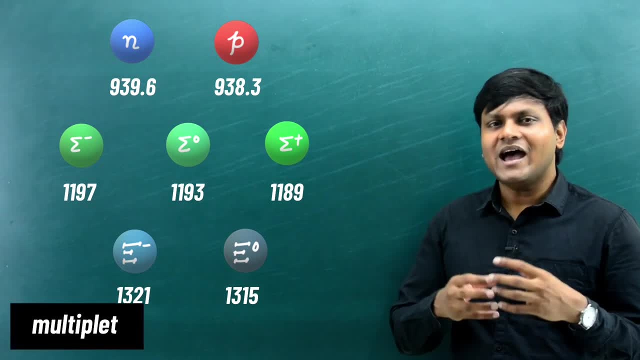 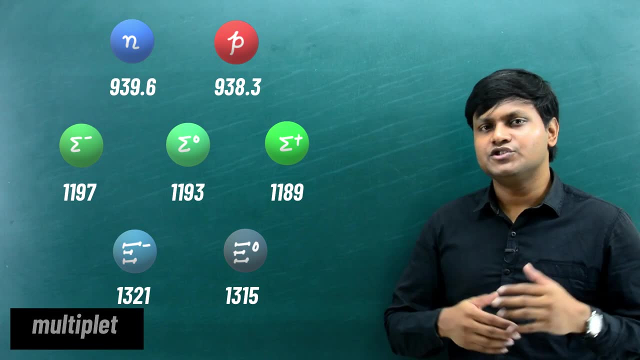 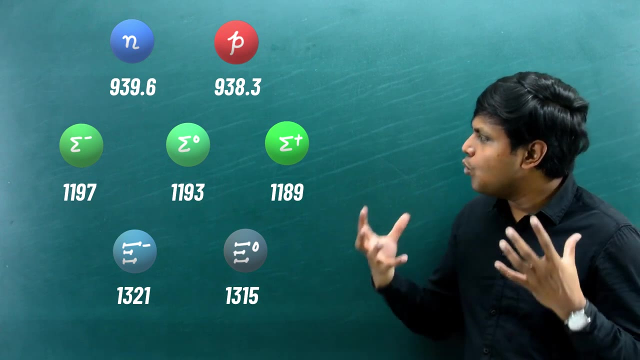 particles, which were organized as multiplets. The idea is that maybe these particles are the result of some fundamental entity having different charge states. Now, in the Eightfold Way, all of these groups of particles were combined in one chart that looks something like this, which is what you 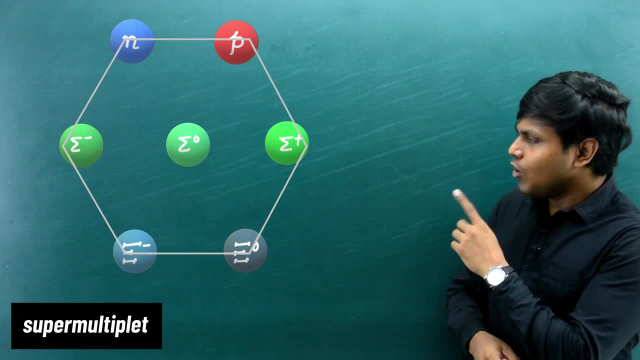 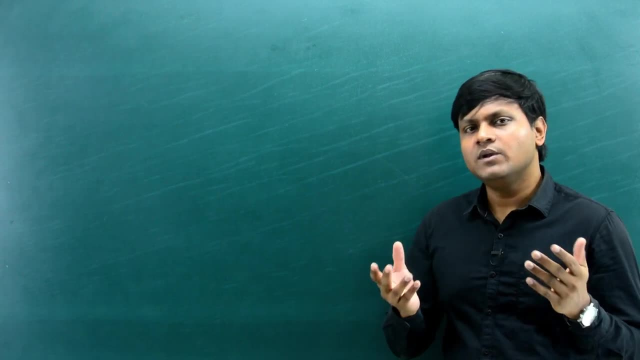 can call a super-multiplet. All right Now, before I talk about this chart in detail, let me first mention that the idea of Eightfold Way is kind of similar to the idea of the periodic table. Now, what is the periodic table? 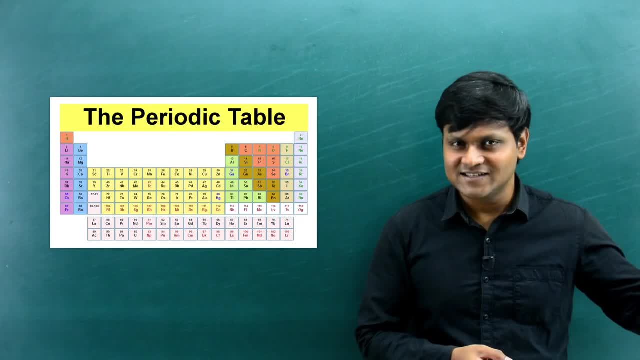 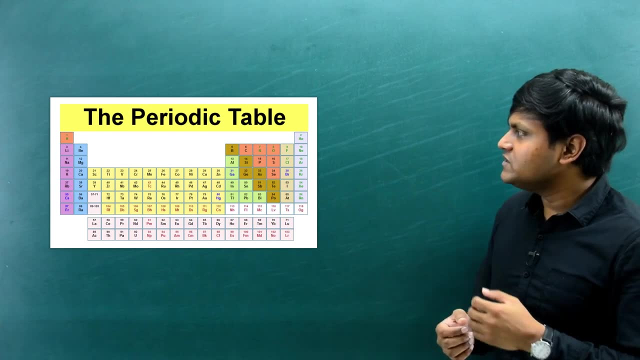 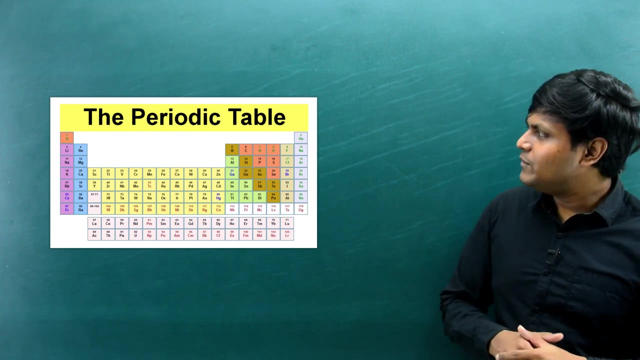 When scientists were studying the chemical elements, the huge diversity of atoms out there, then they tried to organize all the atoms in a particular manner in this particular table, with certain rules, And organizing all the chemical elements in this kind of a chart basically helped us create a 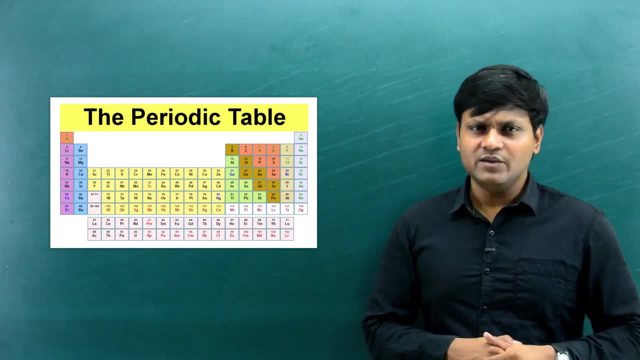 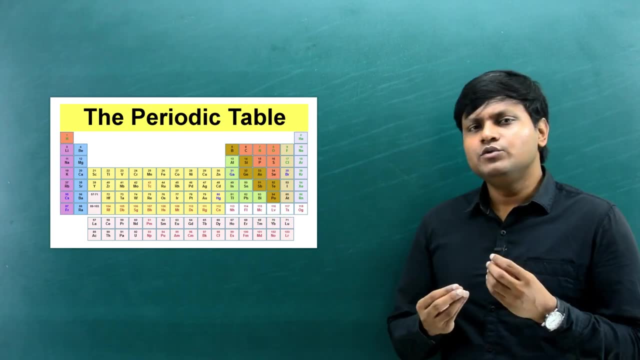 certain kind of order in the chaos and the diversity of chemical elements. It helped us in studying the similarities and dissimilarities between different atoms And also alluded to the fact that all of them are in fact made up of the very same particles, but in different. 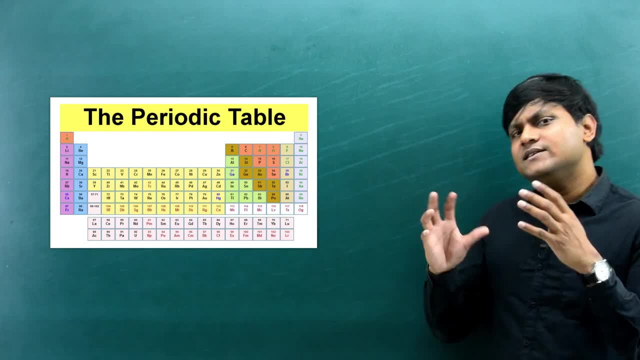 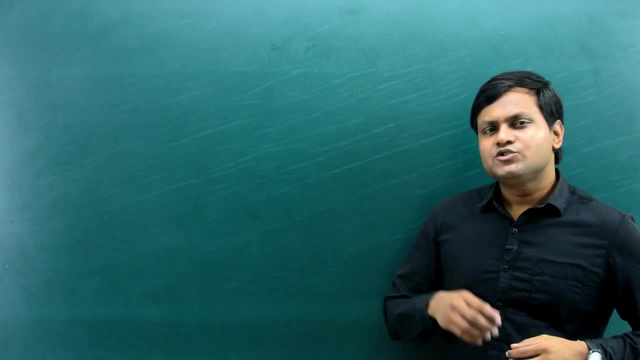 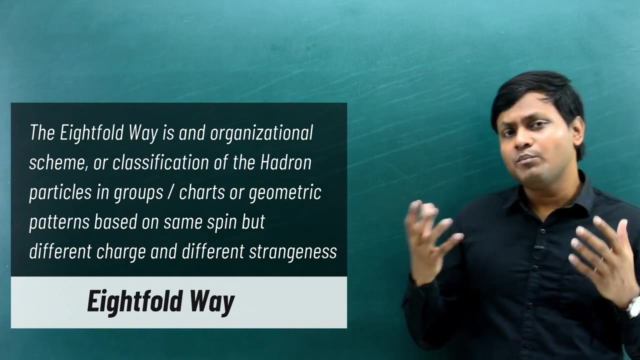 combinations: electrons, neutrons and protons. So the idea of Eightfold Way is similar to that of the periodic table, but for subatomic particles. So the Eightfold Way is in a sense an organizational scheme or classification of the hadron particles in groups or charts. 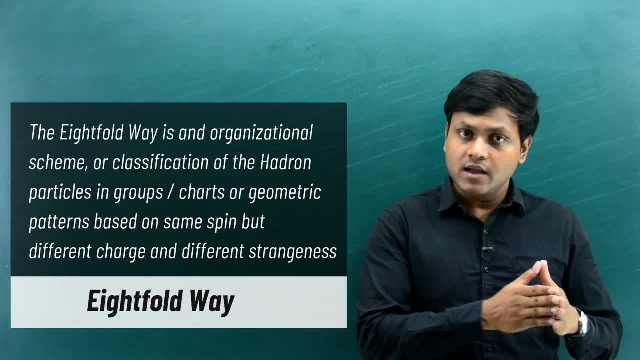 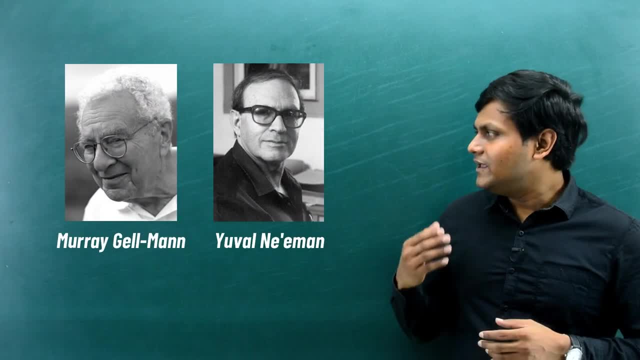 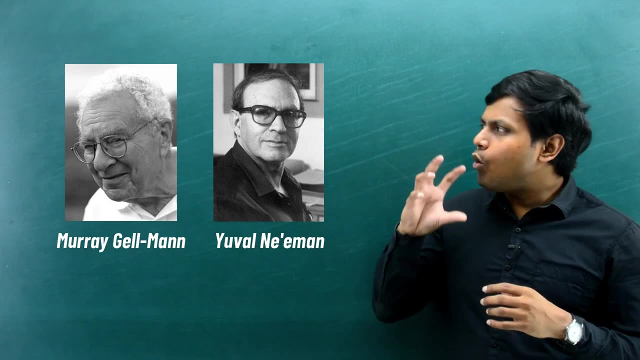 or geometric patterns based on same spin but different charge and different strangeness. It was independently proposed by two scientists, Murray Gilman and Yoval Neiman. They proposed this of eightfold way of organizing all these hadron particles into certain charts, or 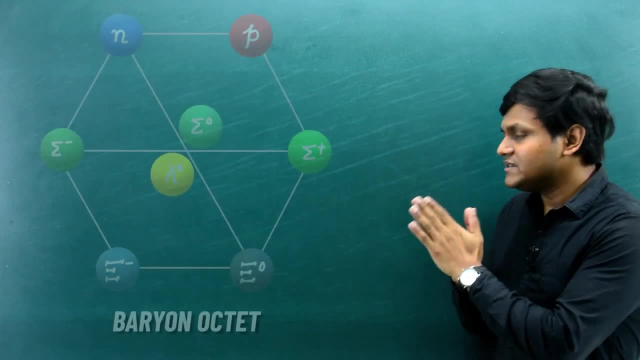 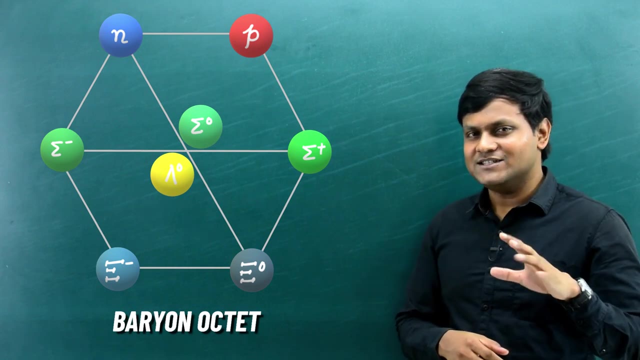 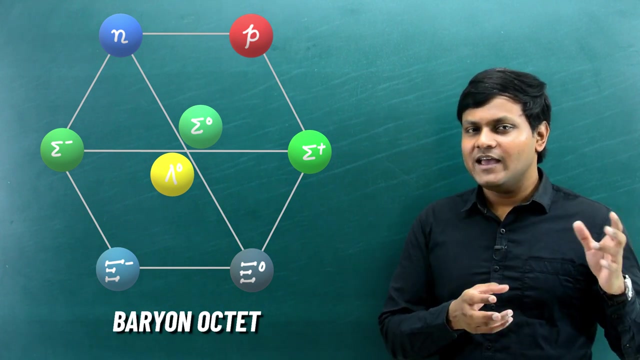 grids or geometric patterns. one of them is this, the baryon octet. so you see here, this chart basically consists of eight particles. you see eight, the name eightfold, so the idea of the naming of the eightfold way, the eight, comes from these eight particles. as it turns out that many of these charts, or grouping of, 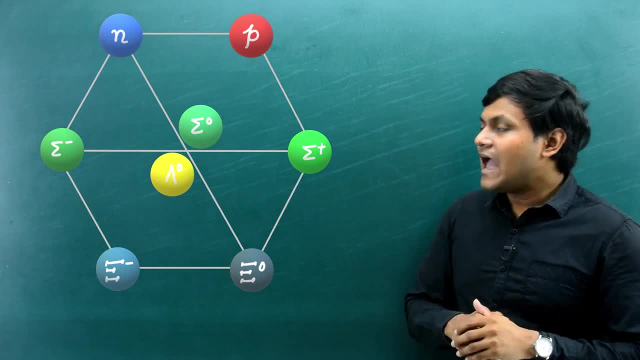 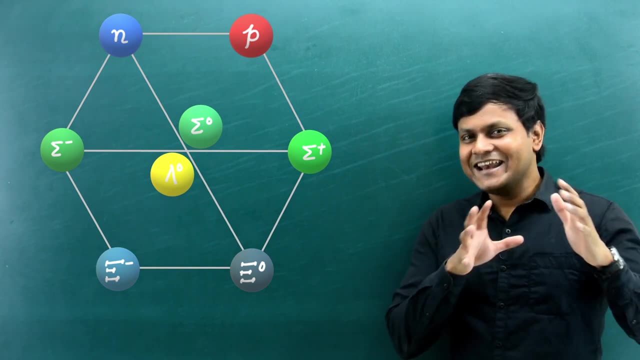 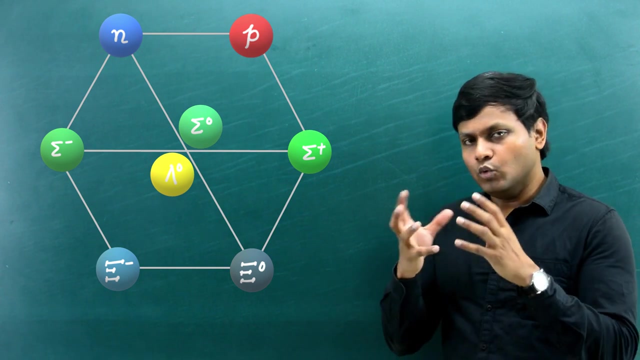 particles consists of eight particles, not all the time. and also, Murray Gilman was inspired by the eightfold pathway in Buddhism. okay, so there is a relation there somewhere. so he was inspired by the idea of eightfold pathway in Buddhism and he used that word of eightfold way in describing the 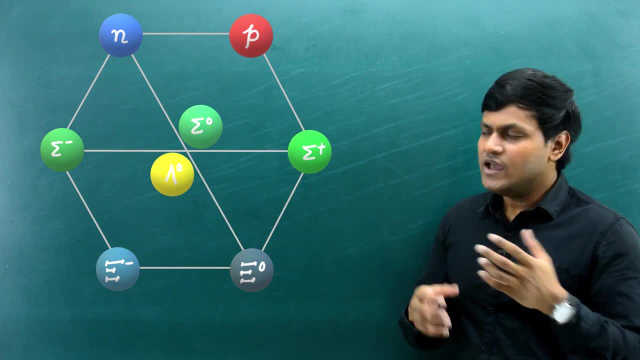 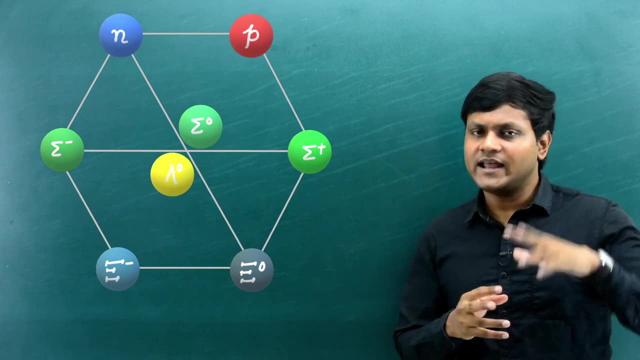 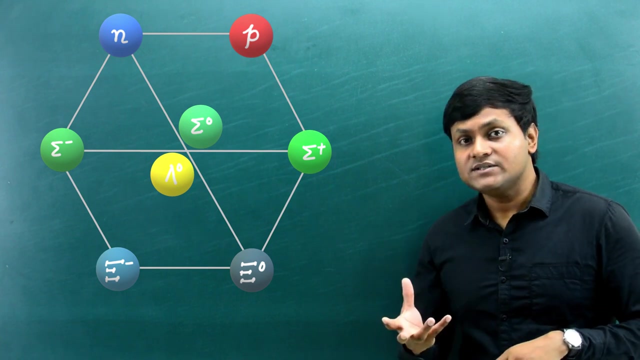 organization of these particles. so let us understand what they actually mean. here we have you the lightest baryon particles. now, what are baryons? when I talked about hadron particles, I said that hadrons can be divided into further two categories. one is the baryon particle and other are the meson particles. baryons are fermion. 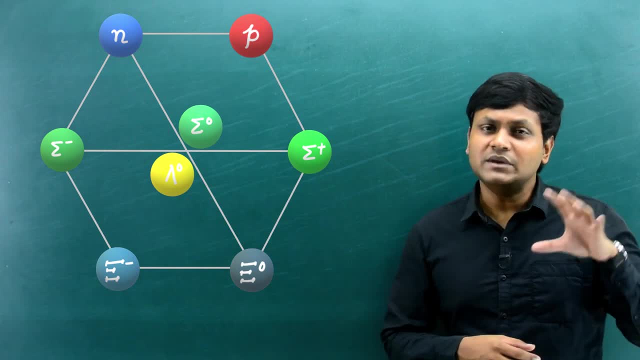 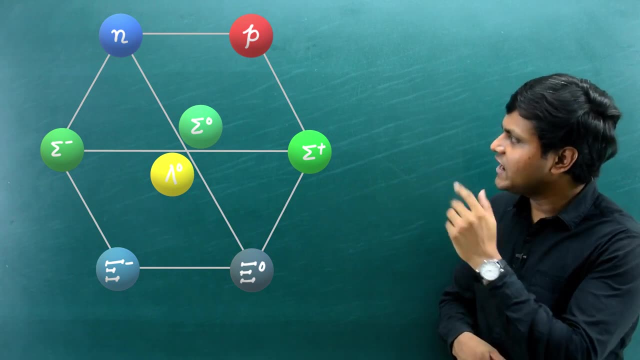 particles. they follow the Pauli's exclusion principle. but mesons are boson particles that do not follow the Pauli's exclusion principle. so the lightest baryons can be organized in this kind of a manner where you have these eight particles: the neutron, the proton, the Sigma plus Sigma zero. 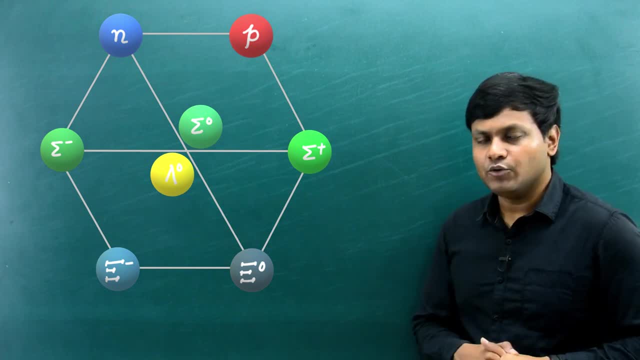 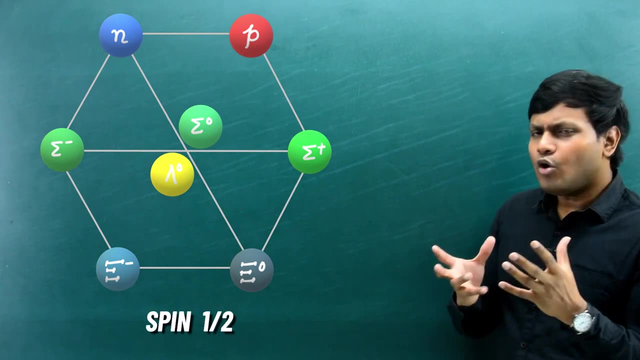 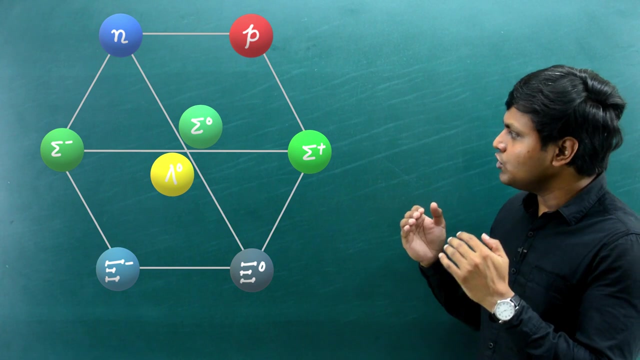 lambda, Sigma minus, and the size. and, as I see now, these are all spin half particles. all of these have spin half. okay, now they are not organized in some kind of a random fashion. there is a logic to this kind of an organization. you can understand this logic by imagining that this geometric pattern is 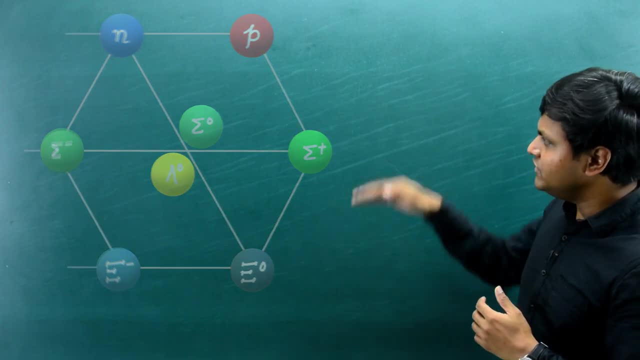 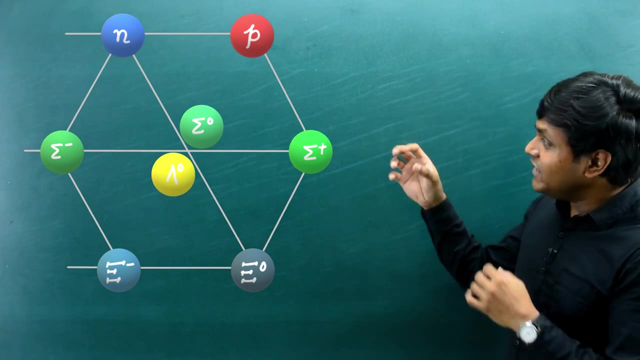 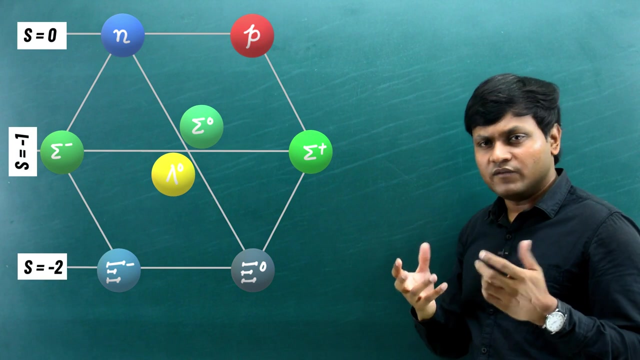 being created by these lines. you have these horizontal lines, okay, and you have these diagonal lines, okay. so there is a particular, you can imagine a grid, a, which ends up creating this kind of a hexagonal pattern. so the top horizontal line represents strangeness, quantum, number of zero. the middle: 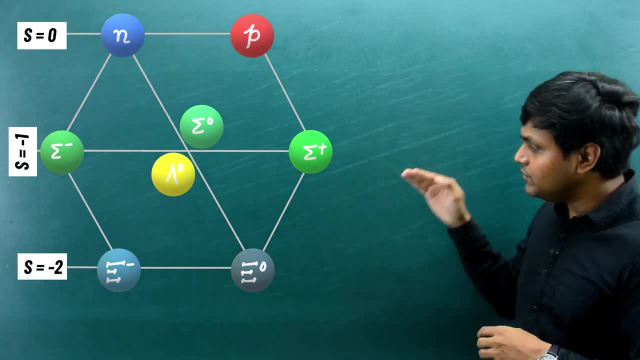 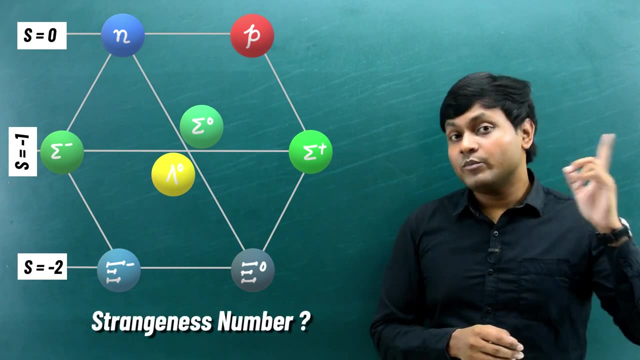 horizontal line represents the strangest quantum number of minus one and the bottom horizontal line represents strangest number of minus two. now, what is the strangest quantum number? again, in one of my previous videos I talked about strangeness quantum number. you see, in the last fifty to hundred years, when 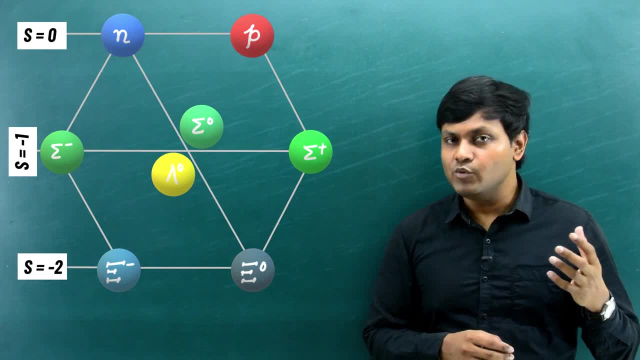 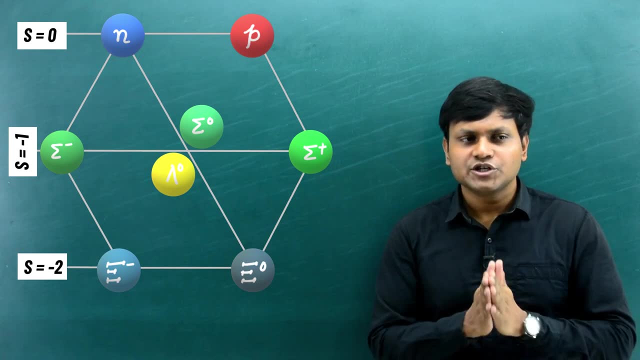 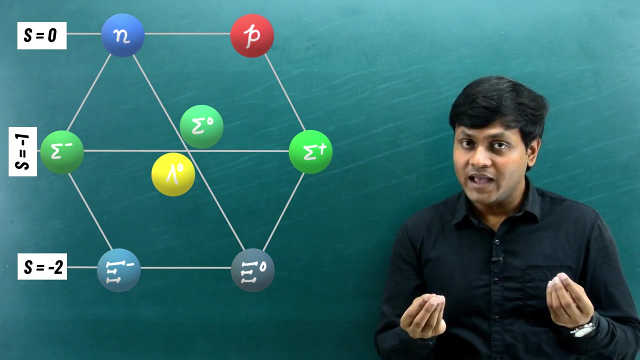 scientists were experimentally discovering newer and newer hadron particles. there is a time at which they found lots of particles which were being created in high energetic particle reactions which seem to behave in a strange manner, and by strange manner I mean that particles were being created by either 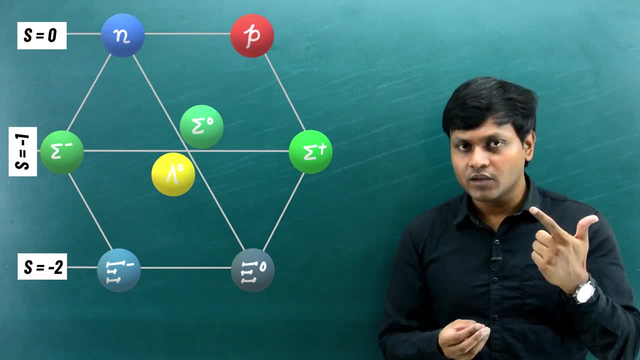 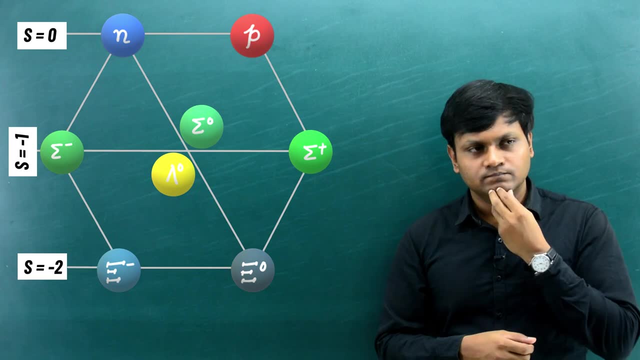 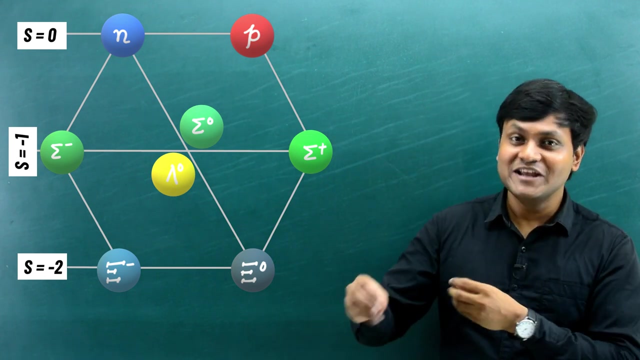 the strong interaction or the electromagnetic interaction, but they were decaying via the weak interaction. so scientists at that point in time thought, hmm, they are behaving in a strange manner. so just because they were behaving in a strange manner, they named those particles as strange particles. hmm, these are behaving as 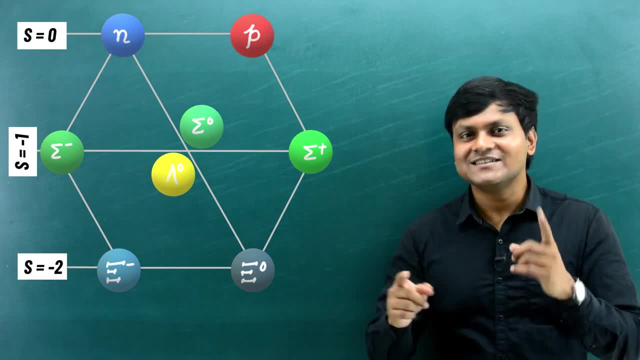 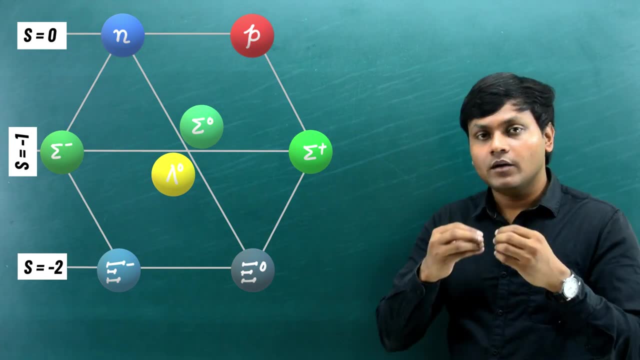 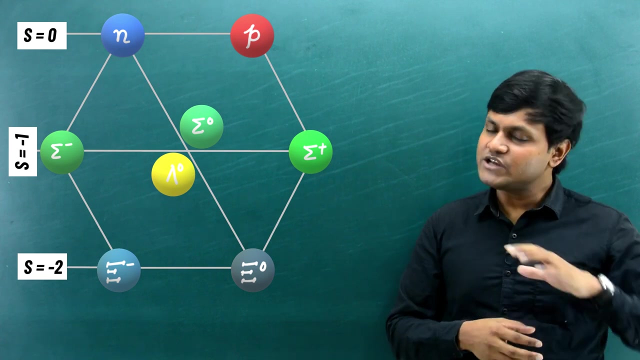 strange particles, so let's name them a strange particle. do you understand the logic of the name? well, that's how particle physicists name particles, and so they therefore came up with a quantum number called the strangeness quantum number, based on how these particles are created and how they decay, which I've 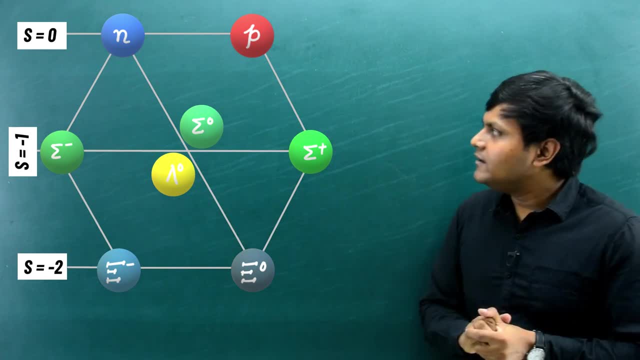 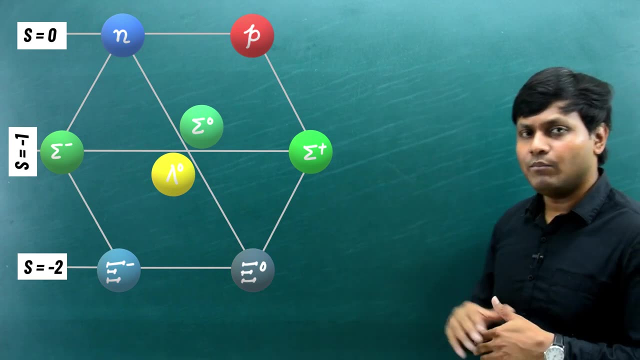 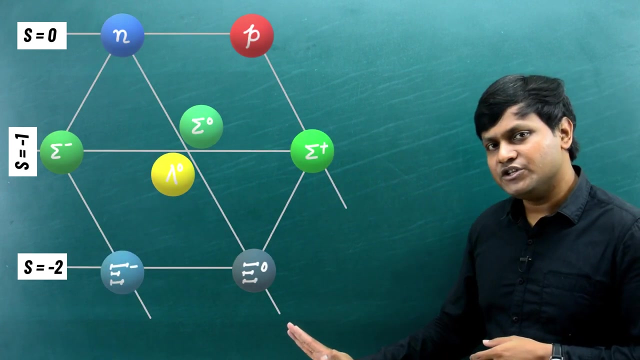 talked about in detail in one of my earlier videos, and this is what the S represents here. it represents the strangeness, quantum number of zero, minus one and minus 2. also, the diagonal lines here represent the charge you have. Q is equal to plus one electronic charge, zero electronic charge and minus. 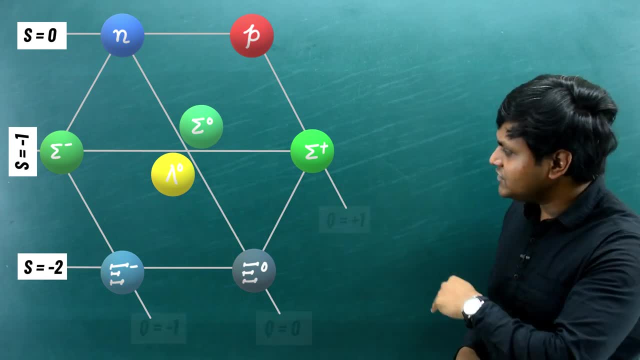 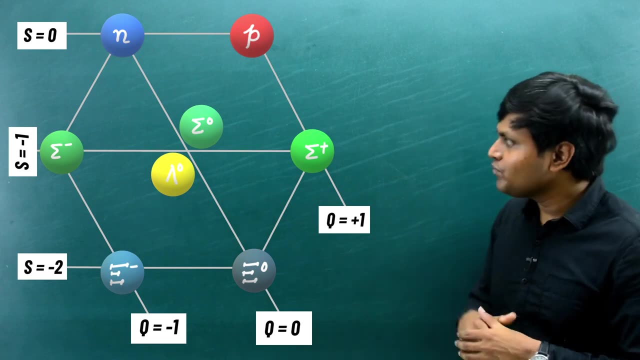 electronic charge. okay, and, as you can see, when these three lines of charges- plus 1, 0 and minus 1- intersect with strangeness of 0 minus 1 and minus 2, at each point you end up getting a hadron particle. so you have the neutron and the proton, which have zero strangeness, but they are not chagrines and they are not negative charges and these are not Özden's characteristics and these are not have charges of 0 and plus 1. all right, you have the sigma plus, which has a strangeness of minus. 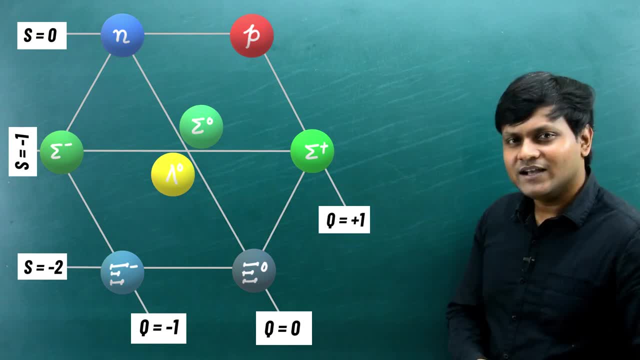 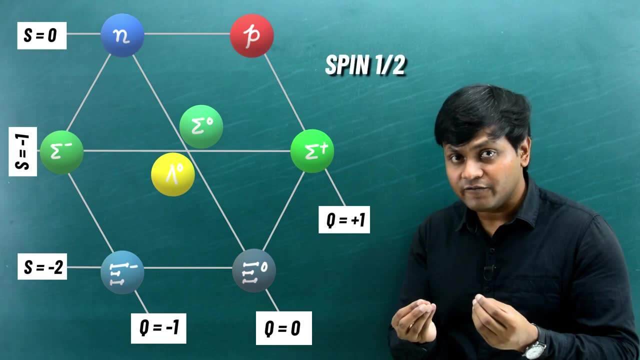 1 but the charge of plus 1. similarly you have the xi particles, which has a strangeness of minus 2. so all these hadron particles, the eight particles which are baryons of spin half, can be organized in this kind of a hexagonal geometric pattern, so essentially they all have same spin of half. 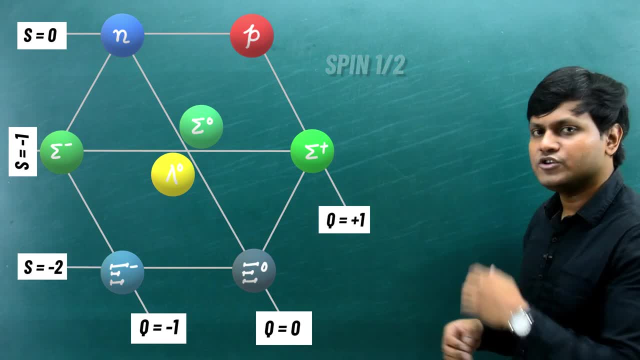 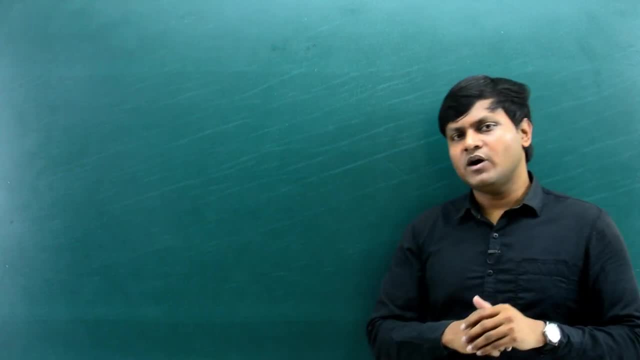 but they are different in terms of their charge, in terms of their strangeness. this is therefore known as the baryon octate. now, this is not the only organization of particles. there are other organizations. so, for example, you have the meson octate, which is another hexagonal organization of 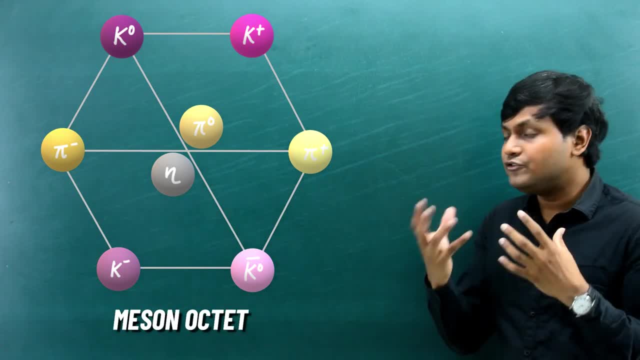 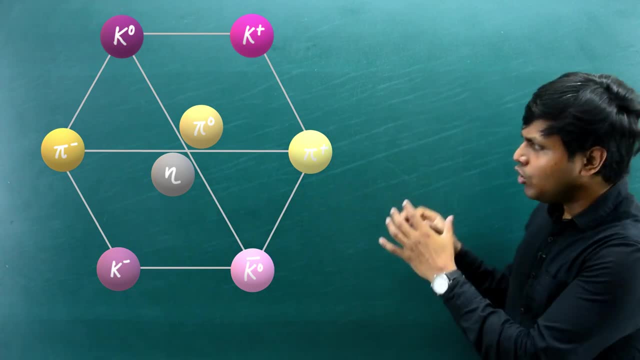 meson particles. so, as i said, mesons are hadrons, which are basically bosons. they do not follow the Pauli's exclusion principle. so you have eight meson particles here, which are organized in a similar fashion, but in this case the horizontal lines represent strangeness of plus, 1, 0 and minus. 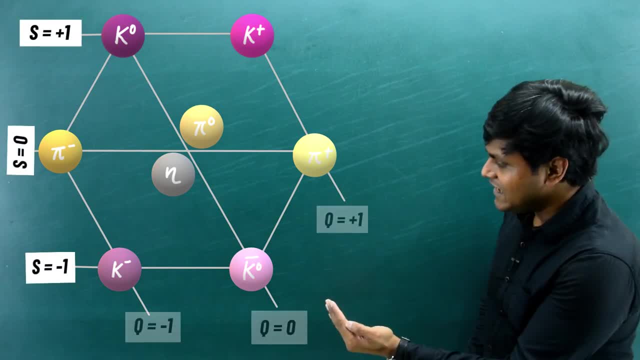 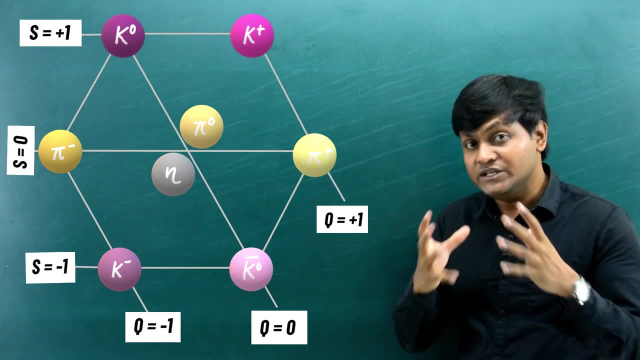 1, while the diagonal lines represent again the same, and you end up getting these eight particles, which are a combination of pi, mesons, eta particles, kaon particles and on and on. these are meson particles that can be placed, and at the intersection of these individual lines now, because they are 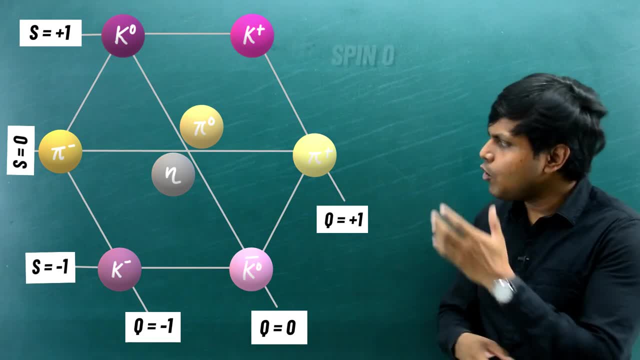 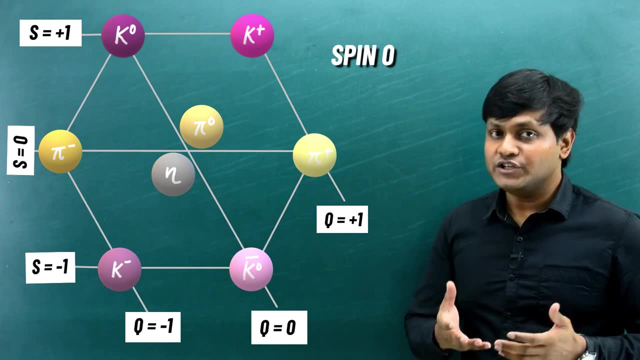 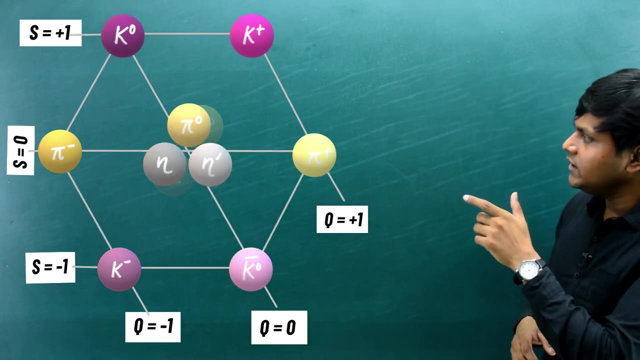 boson particles. they have spin of integer, they all have spin zero. so all these eight particles have zero spin, but differ in terms of their strangeness and electronic charge. now, initially this kind of a classification consisted of eight meson particles, but later on another particle, the eta, prime particle, was added to it. 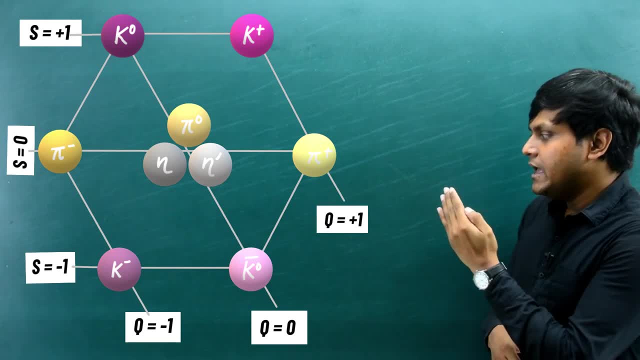 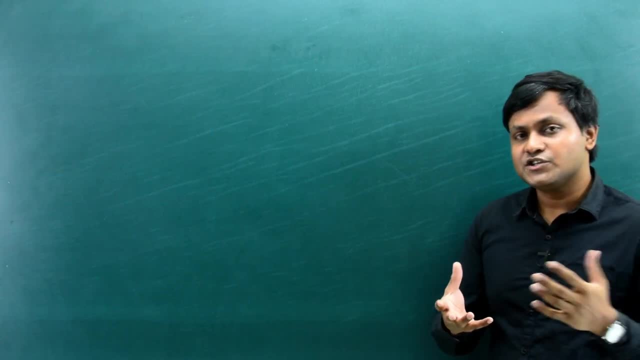 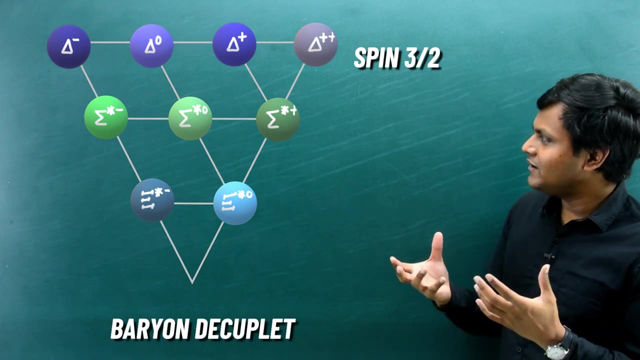 and now, most of the time, this kind of a chart is referred to as a meson nonate, because it consists of nine particles. now there are other organizations of other particles. for example, you have the baryon decouplet, which is not a hexagonal pattern but rather a triangular pattern now. but instead of 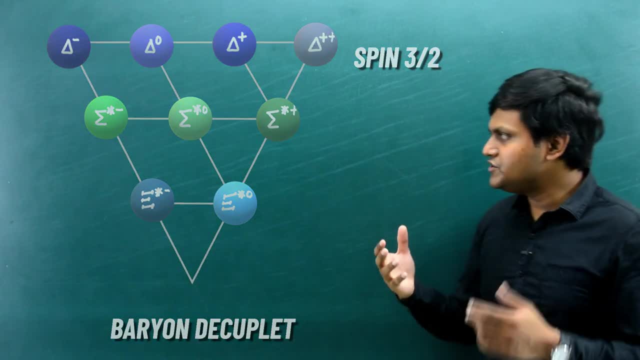 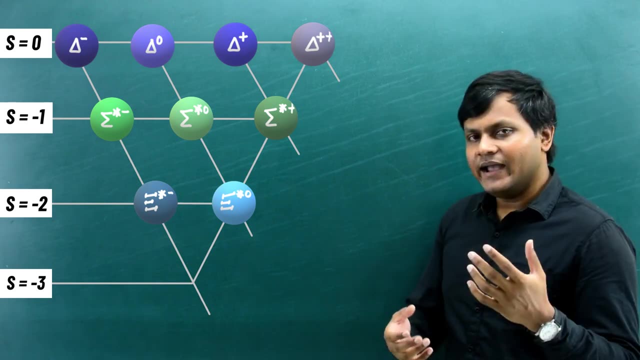 eight particles. it consists of ten particles. so you have the strangeness number represented by the horizontal lines. so you have: s is equal to zero minus one, minus two and minus three, and the diagonal lines represent the charge. you have minus one, zero plus one and plus two. so this is a. 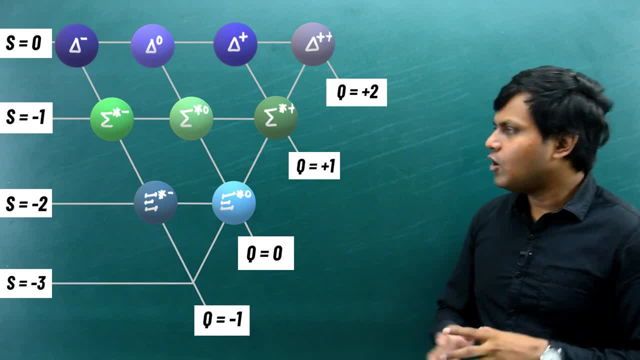 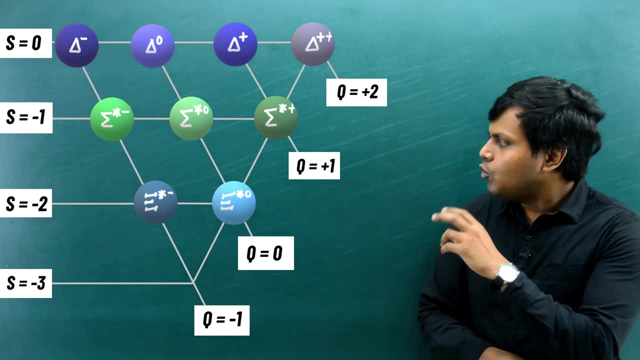 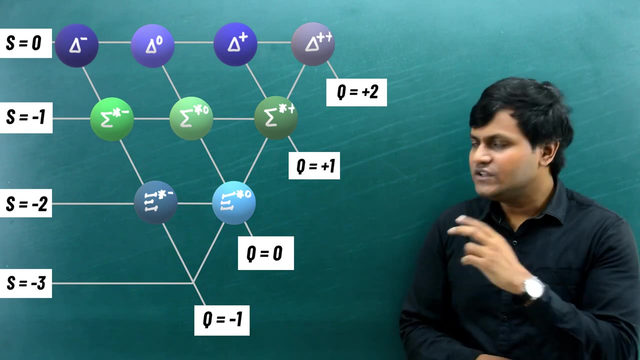 triangular sort of a pattern consisting of ten particles. now, originally, when murray gilman was organizing these particles in these charts or geometrical patterns, only nine out of these ten intersection points were experimentally discovered. nine of these particles were known at that point in time. so what he suggested was that he said that there. 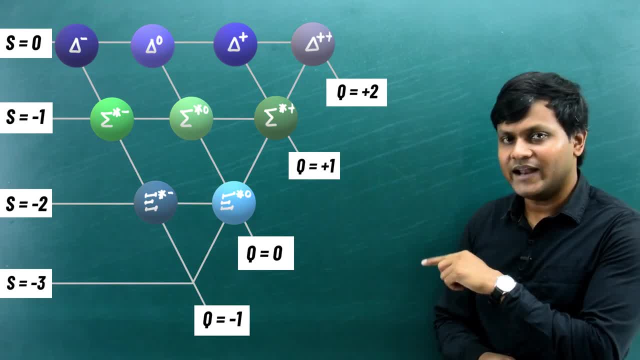 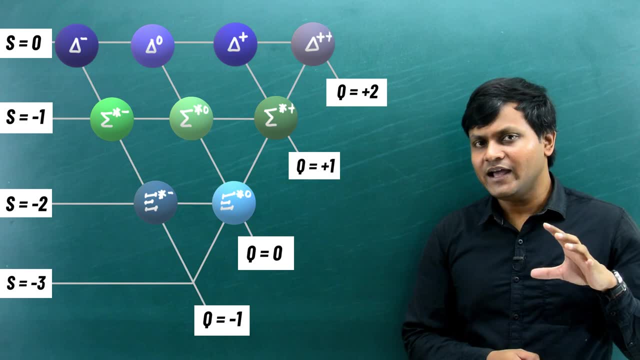 must be a tenth particle. you see the particle at the very bottom that has a strangeness: number of minus three and charge of minus one. that was a particle which was not discovered at that point in time. so, murray gilman, he proposed that there must be a tenth particle having strangeness of. 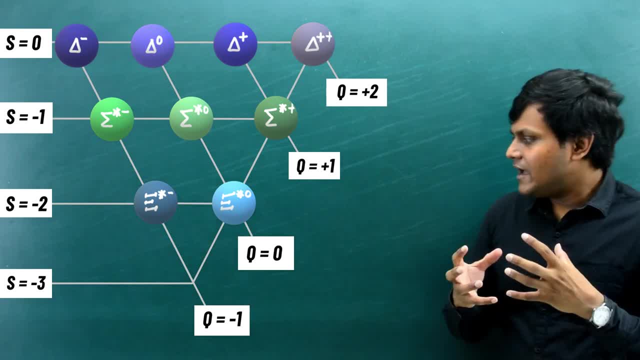 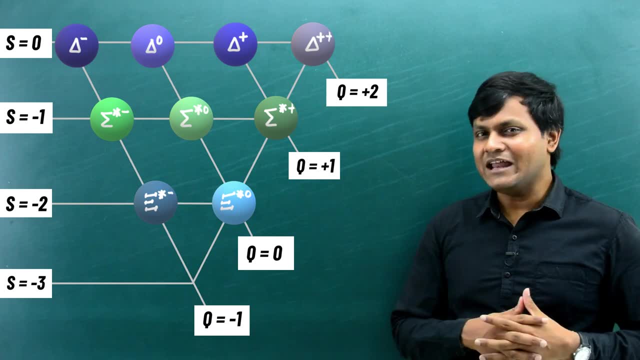 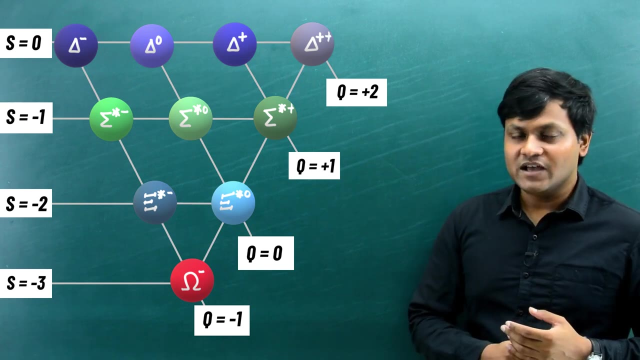 minus three and charge of minus one, and he said that this kind of a particle can be discovered and he suggested the experimental physicists at that time how this kind of a particle can be created. and in fact, in 1964 this very famous omega minus particle was experimentally discovered, thereby giving 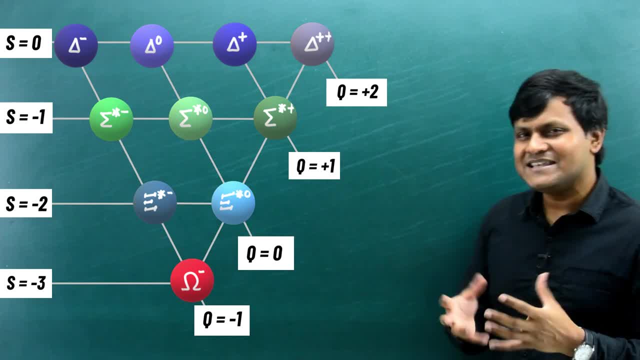 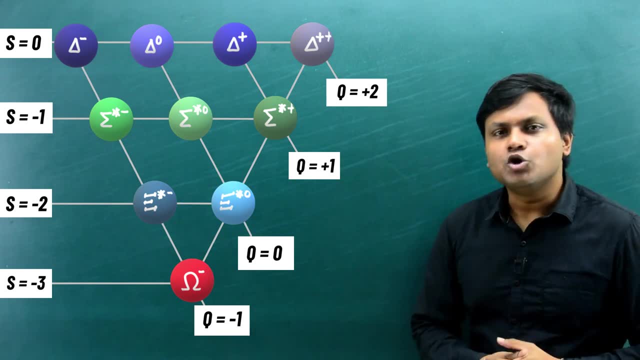 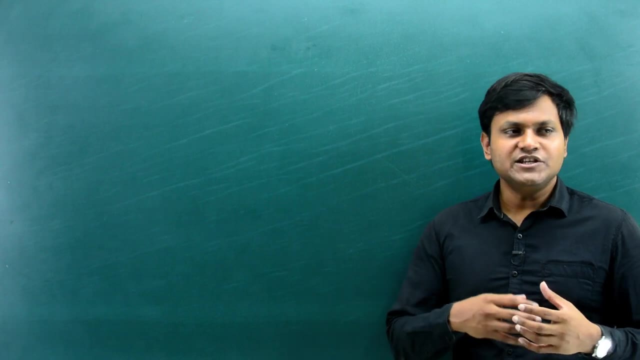 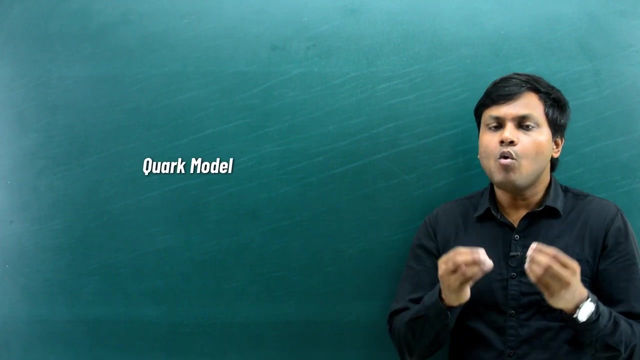 a certain kind of credibility to this kind of an organization of these heteron particles. now, why are we talking about organizing hadron particles in these weird geometrical shapes? this is because the eight-fold way actually was responsible in initiating- uh, you can say- a modern era in particle physics, because it led to the idea of the core model. it predicted the existence of. 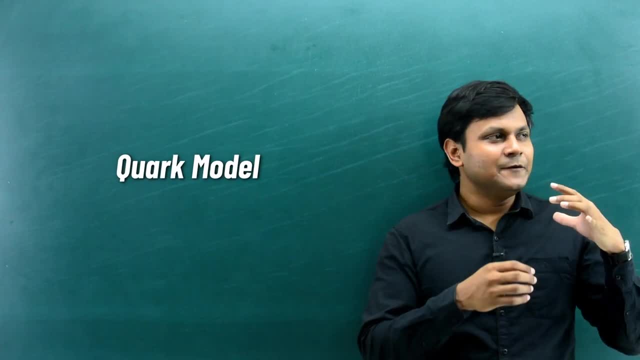 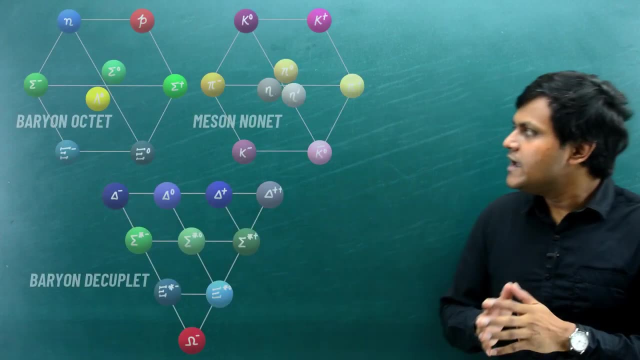 quarks. now, you see, i talked initially about the whether or not these particles are fundamental or are they made up of more fundamental particles? this, this is a very important question right now. if you look at these charts, if you look at the hexagonal form of the eight baryon particles, if 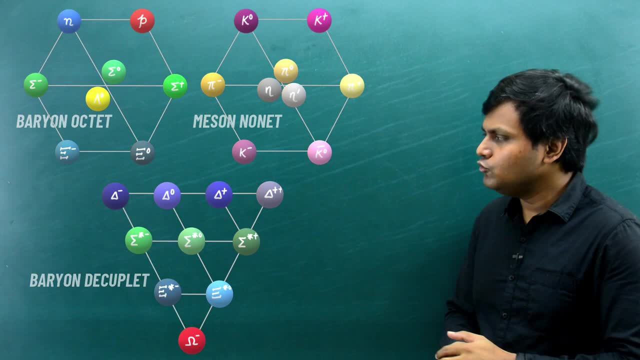 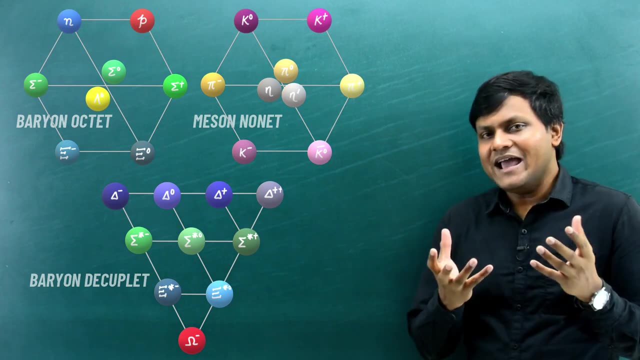 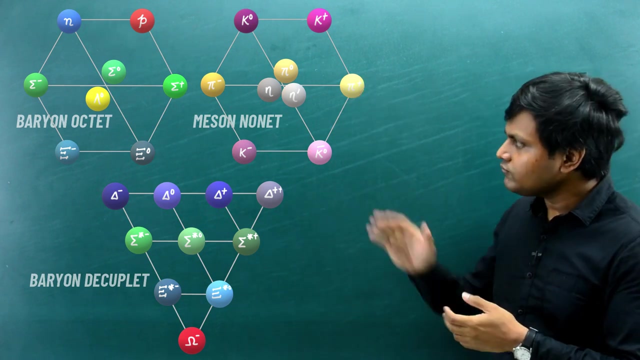 you look at the hexagonal shape of the nine meson particles, if you look at the triangular shape of the ten baryon particles of spin, three by two, then you might feel as if that they all have separate spins. all of them belong to the same spin and they are differentiated by charge and 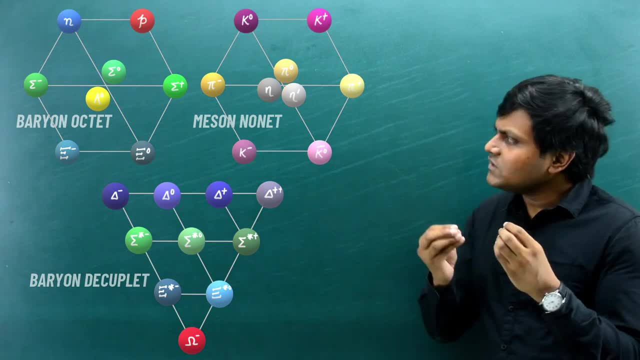 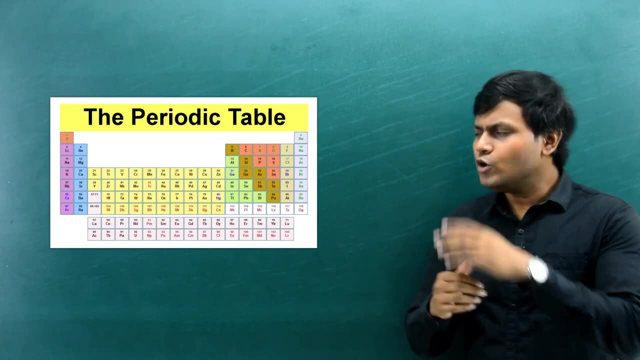 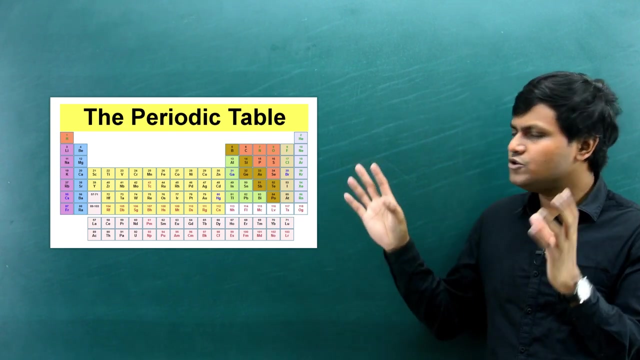 strangeness. so maybe, maybe they might be the result of something more fundamental. okay, here i'm going to talk about, let's suppose, a periodic table. so if you look at the periodic table, all the atoms, uh, having different chemical properties, okay, you have gases, you have solids, you have liquids, you have metals, you have semiconductors, you have insulators. 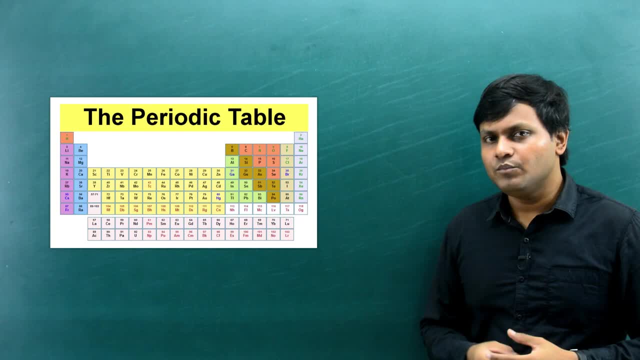 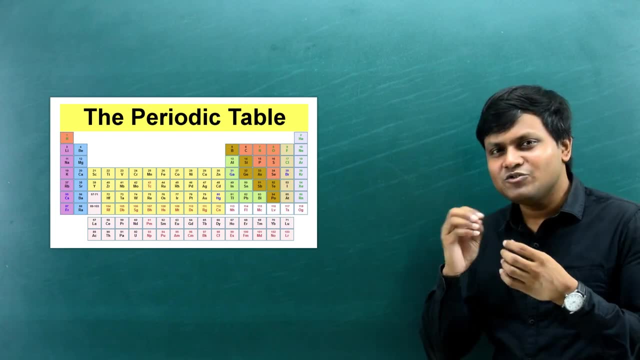 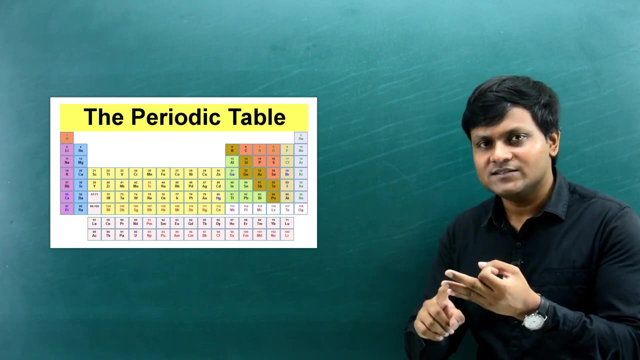 all this vast majority or vast diversity of chemical properties are fundamentally the result of water. they are the result of a few particles combining in different numbers. you have the electron, you have the proton, you have the neutron. these are the particles that combine in different numbers to create these chemical elements and this diversity of properties. 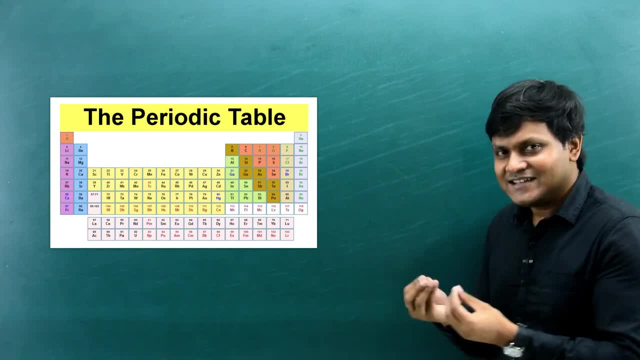 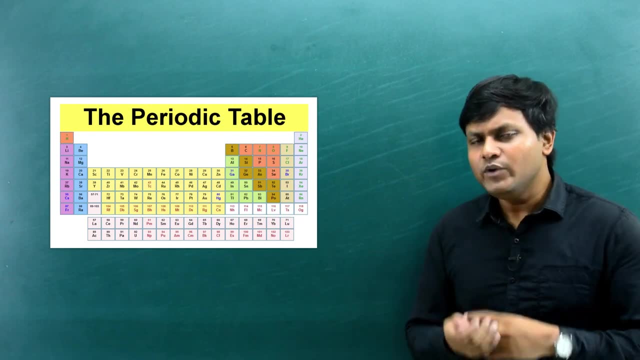 is basically a series of particles and if you look at the periodic table, you can see that there is a series of particles, but they are not different, but the same way that the entire period table is in a sense created by these three fundamental particles, organized in different. 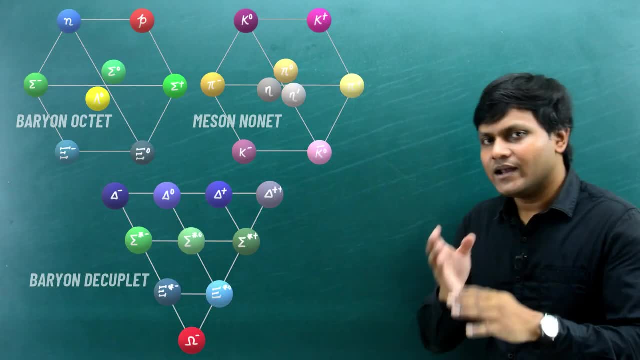 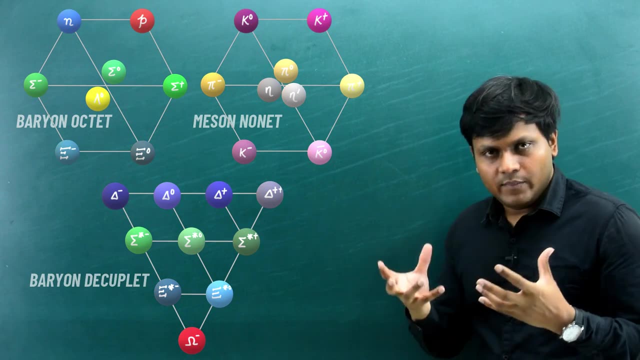 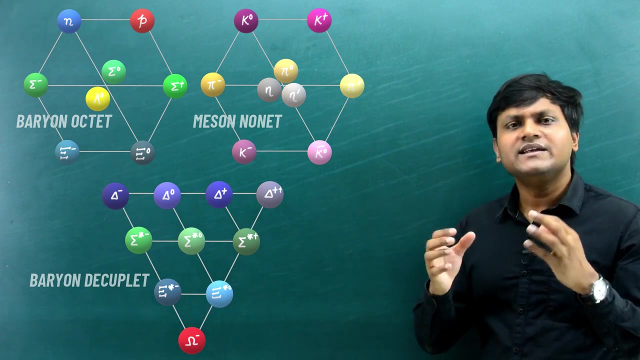 combinations to create this diversity. we can think of it in the same way, in the eight-fold way of classification, that maybe these classification of particles, there are other, furthermore, classifications of other particles also- we'll not discuss too much into it- which, when they combine or recombine in different proportions, ends up creating this vast diversity. 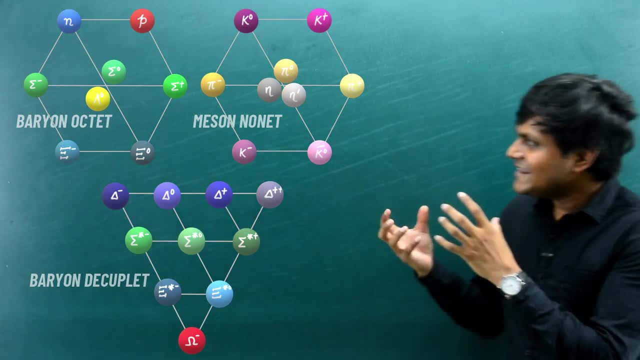 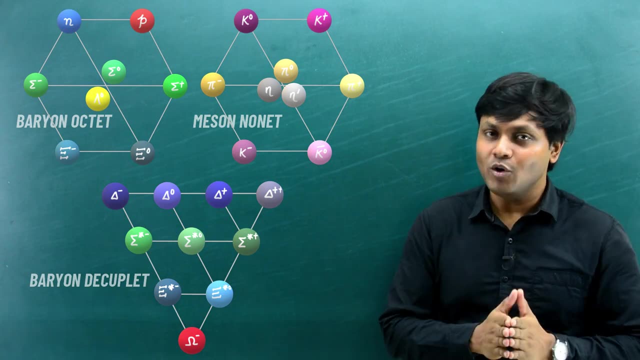 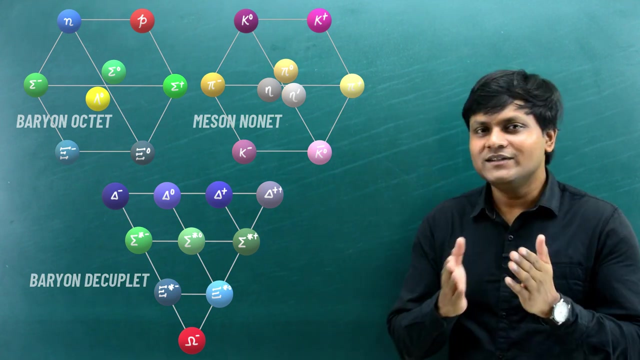 of properties and vast diversity of particles. So in a sense, this eightfold way led to the proposition of what is known as the quark model. So Murray, Gelman and Zweig, they proposed what is called the quark model. What does it mean? So what they propose is that all these particles, they said, 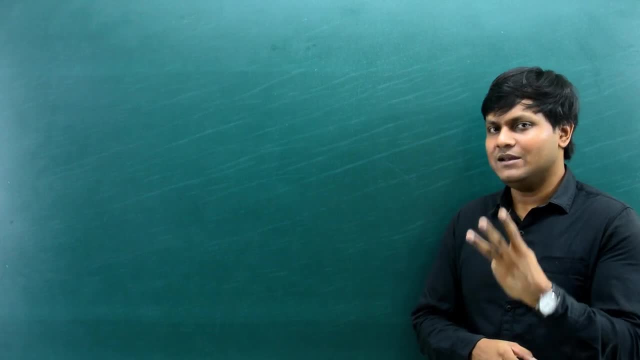 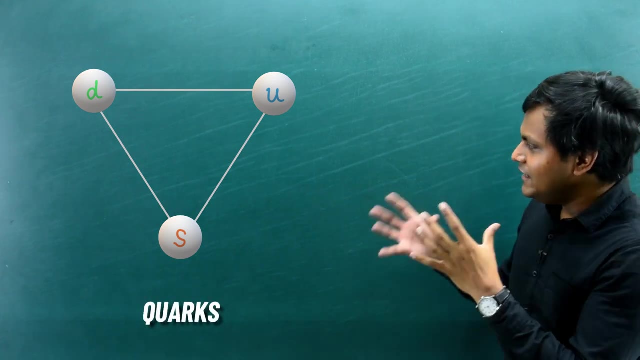 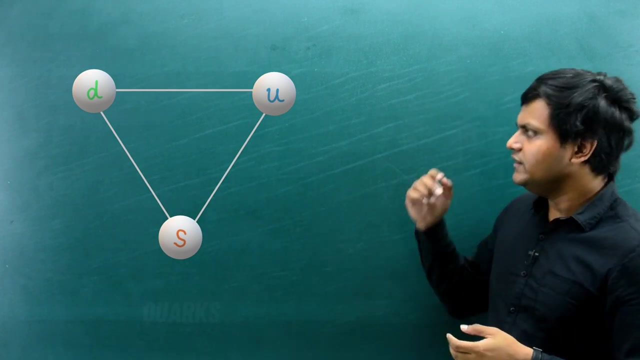 are essentially made up of three fundamental particles, which they called quarks. So you see, here this is the- what you can say- triangular, eightfold way, organization of quarks. Okay, so Murray Gelman said that there are three quarks. You have the down quark, the up quark and the 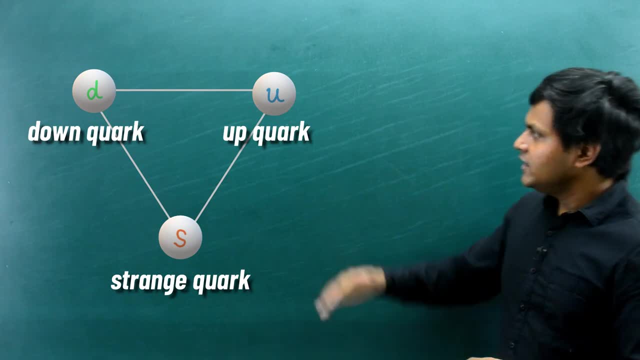 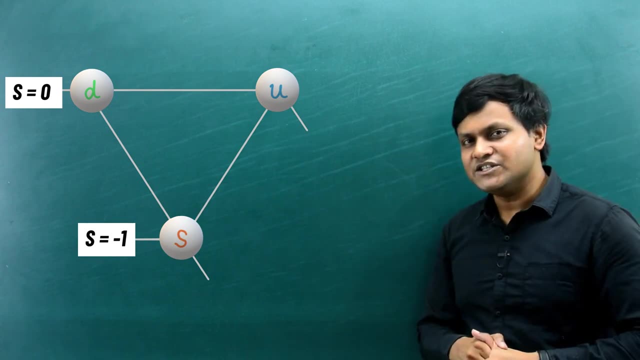 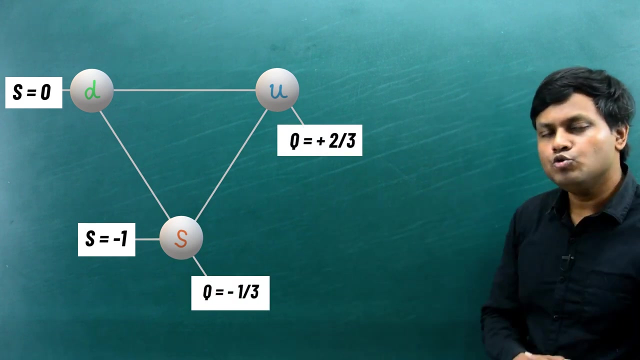 strange quark that can be organized in this kind of a manner. So the horizontal line above represents strangeness of zero, The horizontal line below represents strangeness of minus, The diagonal line represents charges of minus one by three, electronic charge, and plus two by three. 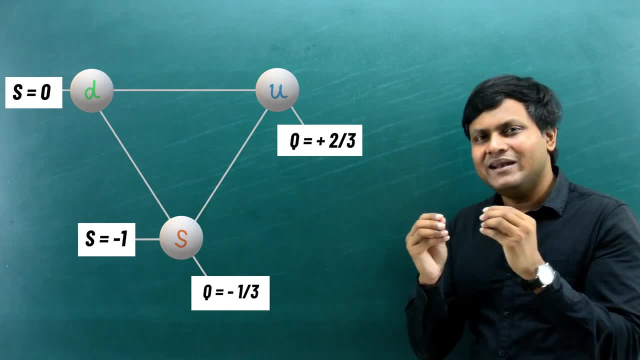 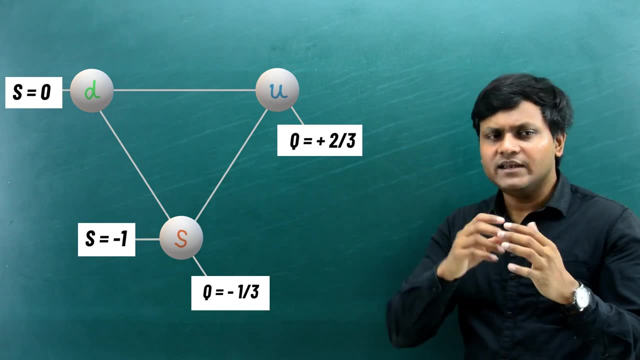 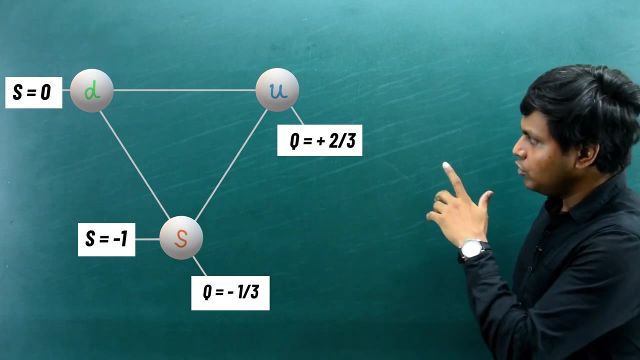 electronic charge. So he said that these are the fundamental entities called quarks: The down quark, the up quark and the strange quark which, when they combine in different manner, ends up creating those hadron particles that we just now talked about. Now one peculiar thing about these quarks: 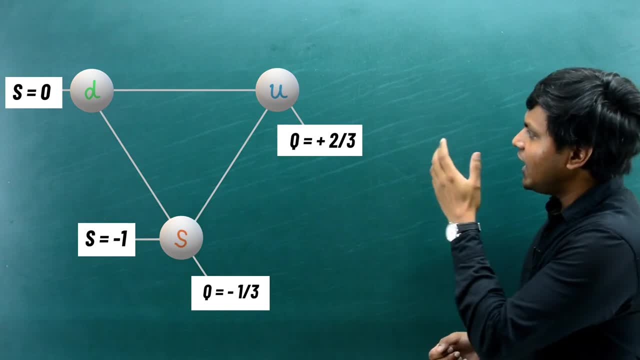 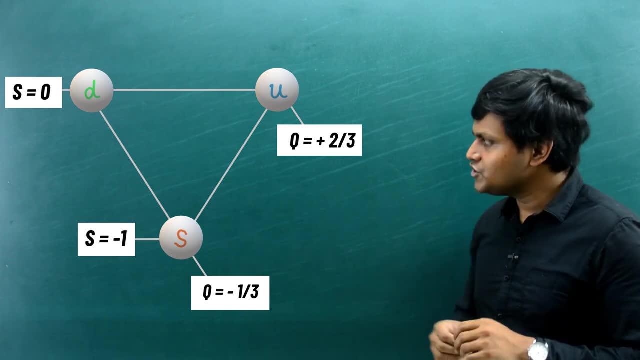 these supposed fundamental particles is the idea that they are all made up of three different matter. The deep plate energy is just the core which chemotherapy can use at this time. The last idea that we totally forgot was about the idea of fractional charges. You see here the up. 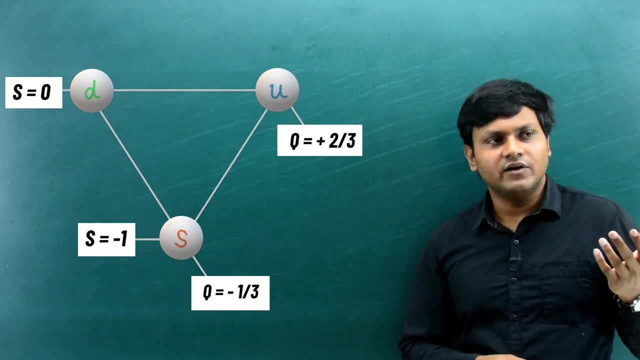 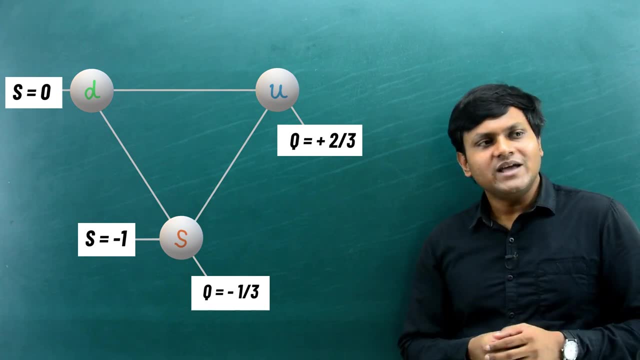 quark has a fractional charge of plus two by three electronic charge, while the down quark and the strange quark has a fractional charge of minus one by three electronic charge. Now, at that point in time, people had not yet discovered three particles that have fractional charges. Even today, 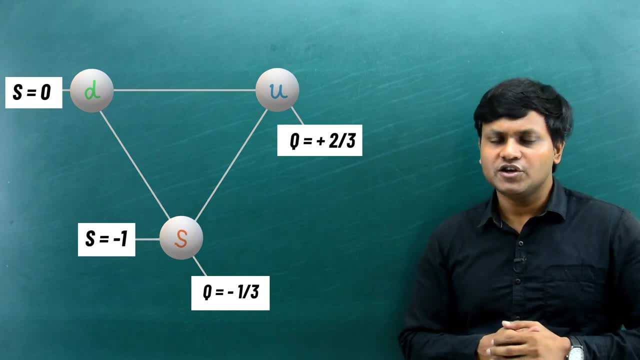 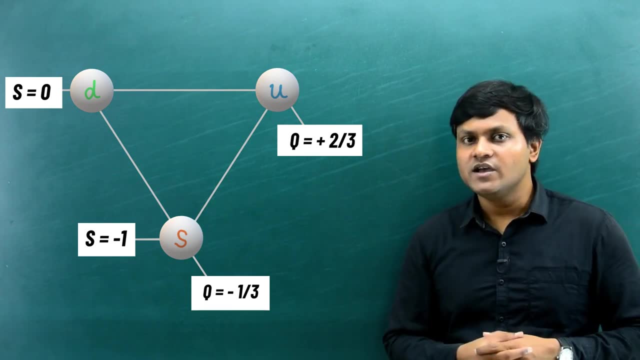 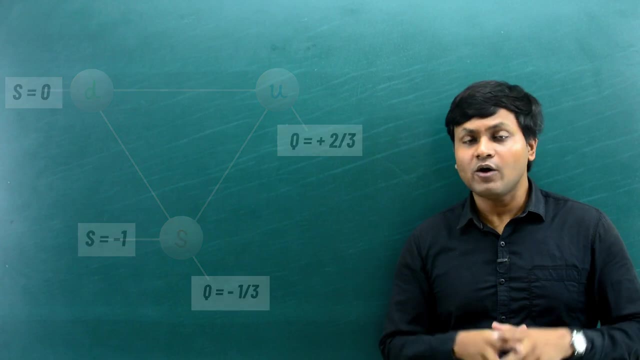 we have not yet found three particles having fractional charges. this idea of fractional charges. however, gelman suggested that maybe these particles, they are always in a bound state inside these hadrons, they are never free from these hadron particles, they are always bound inside these hadron particles. and also high energetic scattering experiments. 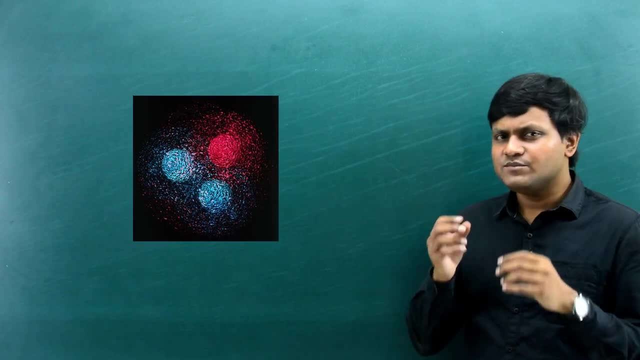 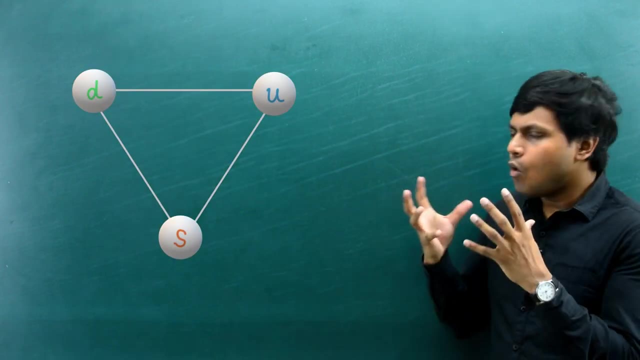 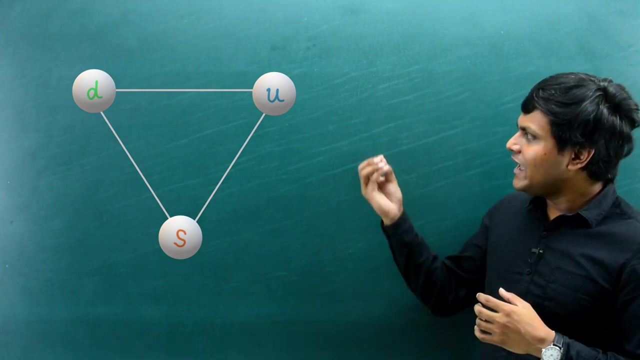 of protons suggested that maybe the proton is made up of three point mass objects and over time this kind of an idea got acceptance. that quarks became a very much sensible idea of explaining this kind of an organization. and by looking at these quarks, their strangeness and their charges, we can easily 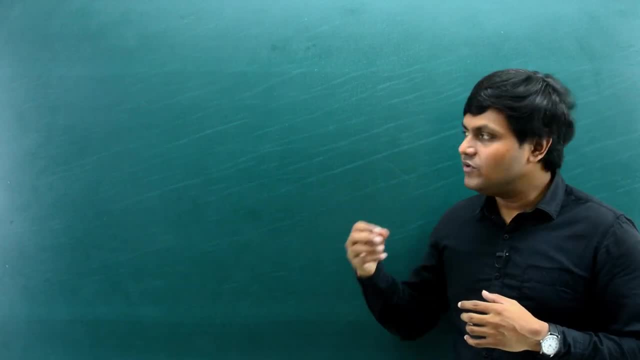 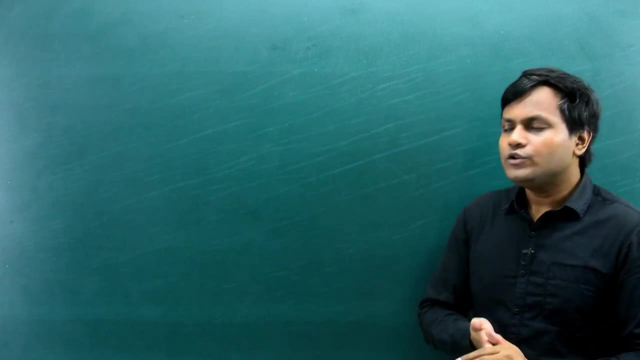 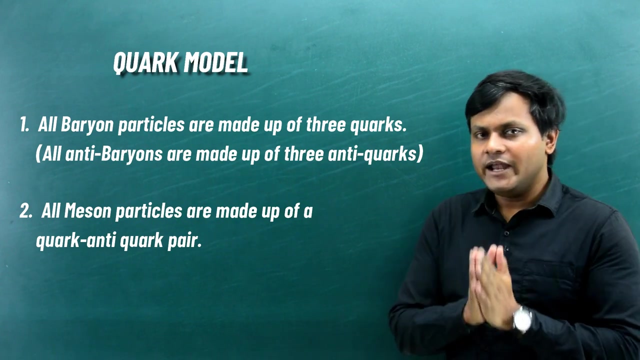 look at these previous charge or previous hexagonal diagrams and see how they are made up of a combination of these particles. so the quark model suggests what it suggests two things. first of all, all baryon particles are made up of three quarks. similarly, all antibaryon particles are made up of three. 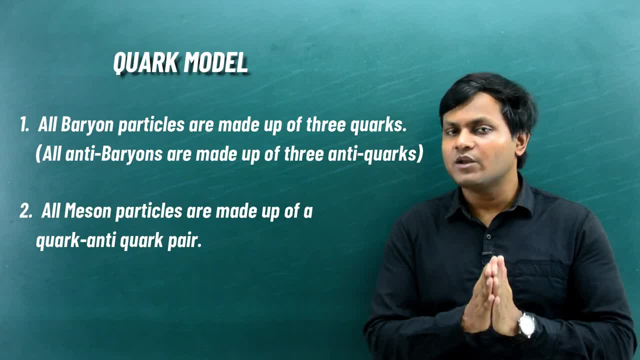 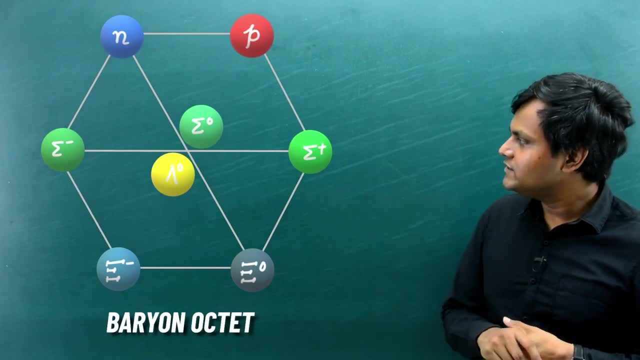 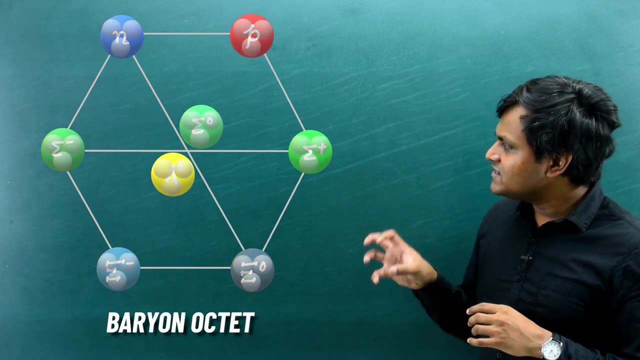 antiquarks. and second, all meson particles are made up of a quark antiquark pair. based on this idea, we can reorganize, let's suppose, the baryon octet. so you see, the baryon octet, which consisted of eight hadron particles, can all be thought of as consisting of three individual quarks inside them. 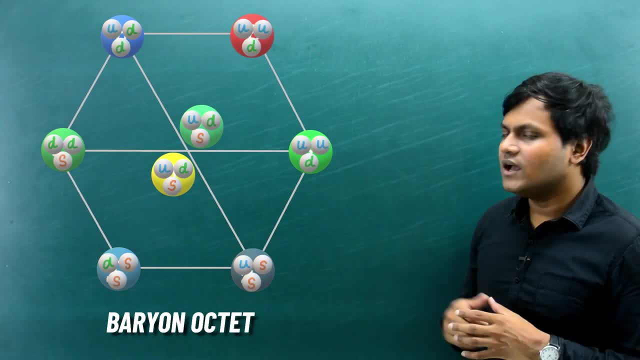 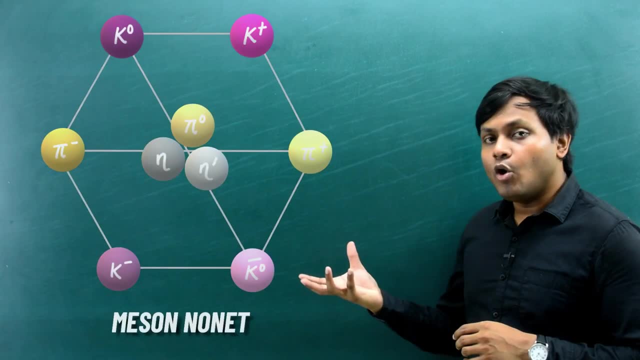 all reorganized in manner. so, for example, the neutron consists of two down quark, one up quark. the proton consists of two up quark, one down quark. similarly, meson nonet can also be thought of as being consisting of nine particles which are individually. 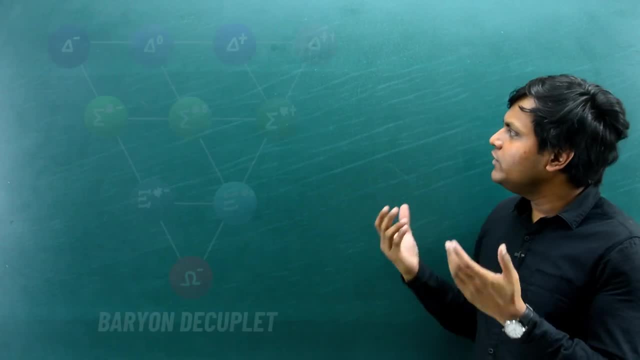 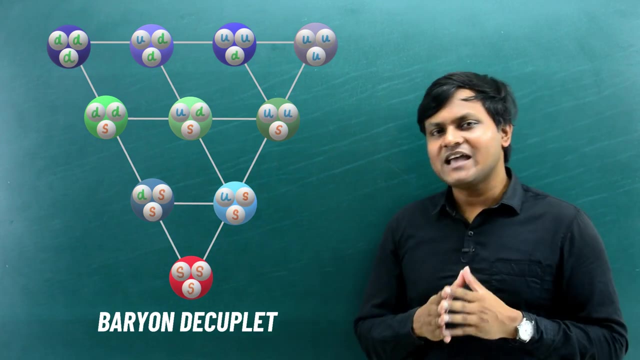 made up of a quark- anti-quark pair, and similarly, we can also show that the baryon decouplet is also made up of ten particles, each made up of three quarks each. now, the interesting idea of this kind of a quark model is that we can 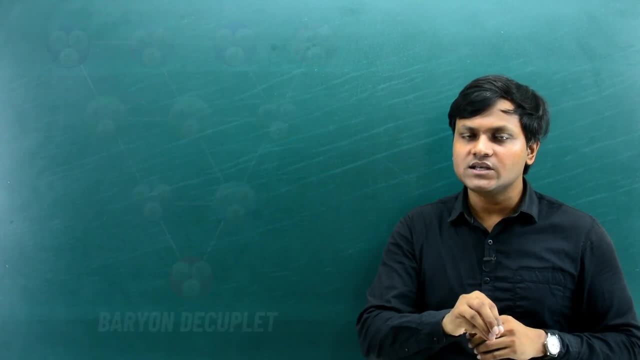 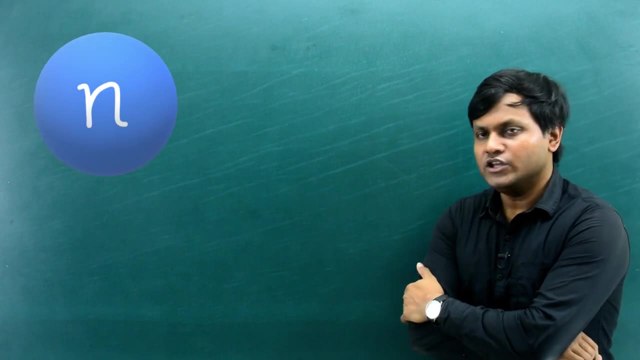 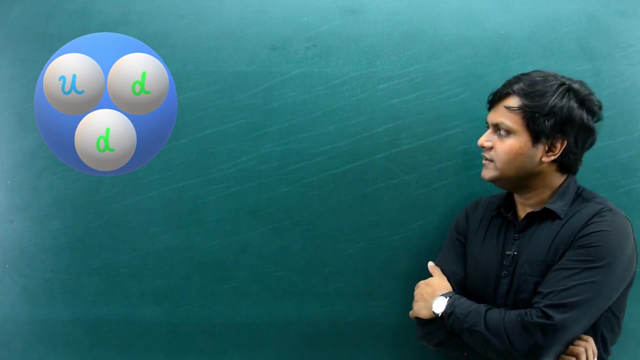 explain the properties of these individual hadron particles based on the properties of the quarks that make them up. so, for example, if you look at the neutron particles, so the neutron consists of one up and two down quarks. so the up quark has a charge of plus two by three and the down quarks has a 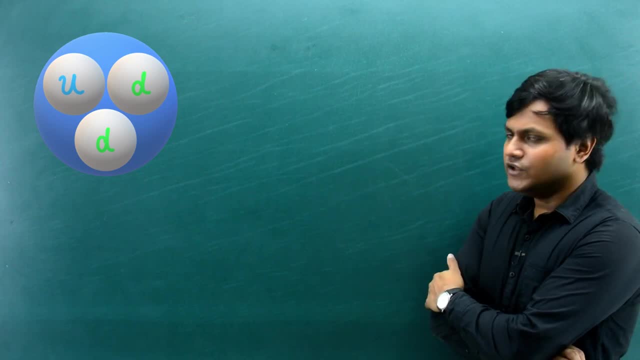 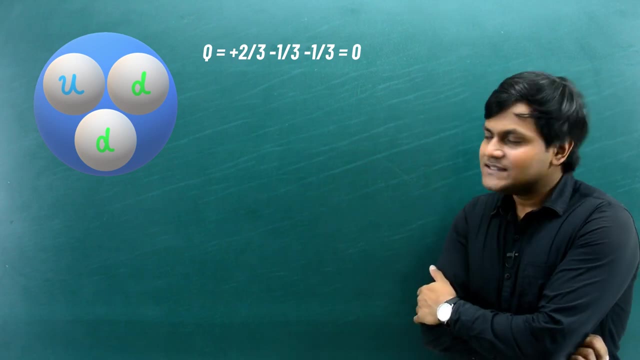 charge of minus one by three. so if you add up the charges of the neutron particle plus two by three, minus one by three, minus one by three turns out to be zero. so the neutron is electrically neutral. similarly, the quarks have spin half. you can organize the spin half of these three quarks in such a: 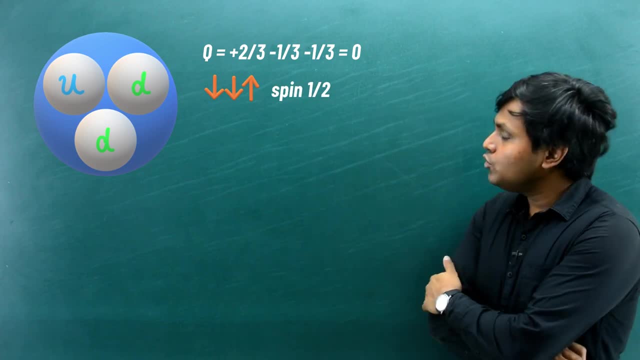 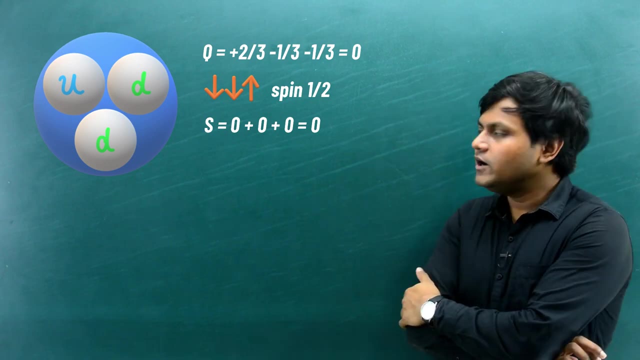 manner that the neutron turns out to also have spin half, also the up and the down quarks of strangeness of zero. so the neutron also has a strangeness of zero. it is not a strange particle. similarly you can also take a look at the proton particle, which consists of two up and one down quark. so basically, 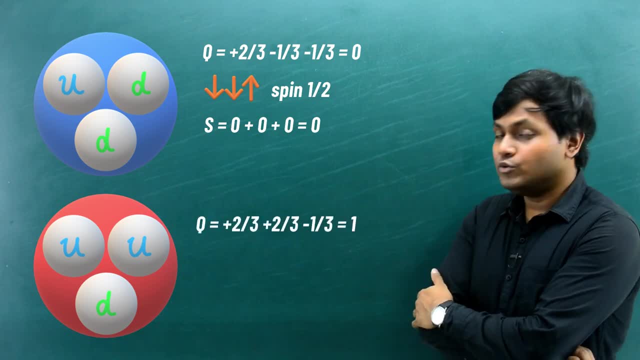 its charge must be plus two by three, plus two by three, minus one by three, which is plus one. so the proton is plus one electronic charge. it is also spin half particles, because three quarks are coming together. so that's why the neutron is also a spin half, because three quarks are coming. 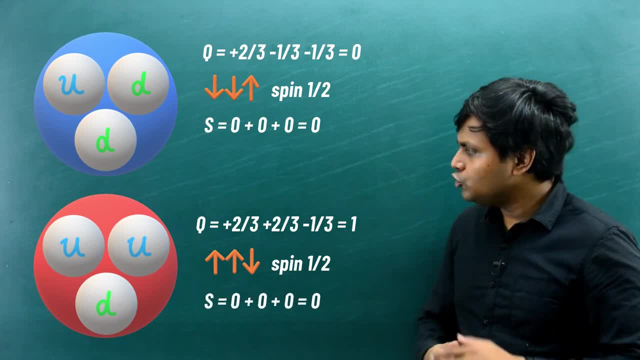 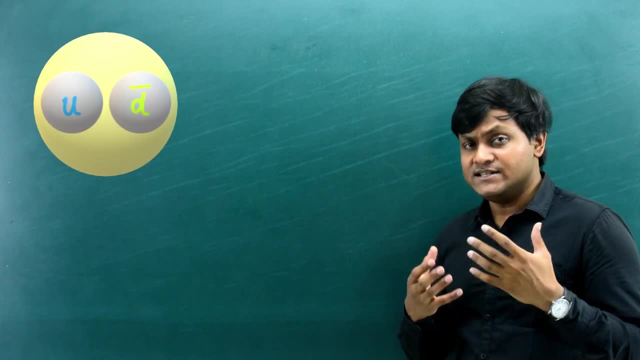 together in this kind of a fashion, and its strangeness also comes out to be zero. If you look at a meson particles- let's suppose a pi meson, a pi plus, which is made up of a up and anti-down quark- then it seems to have a charge of plus two by three, plus one by three, which is 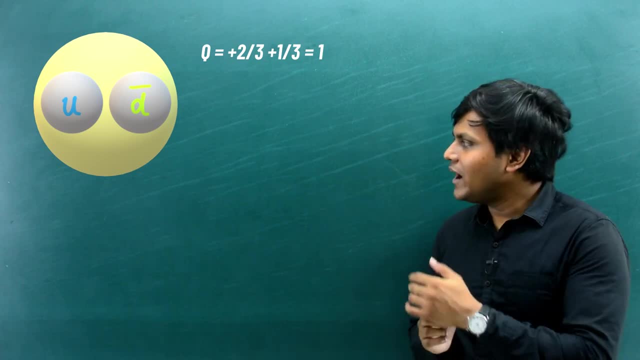 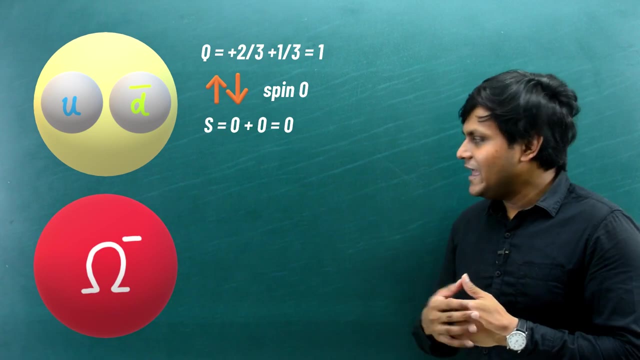 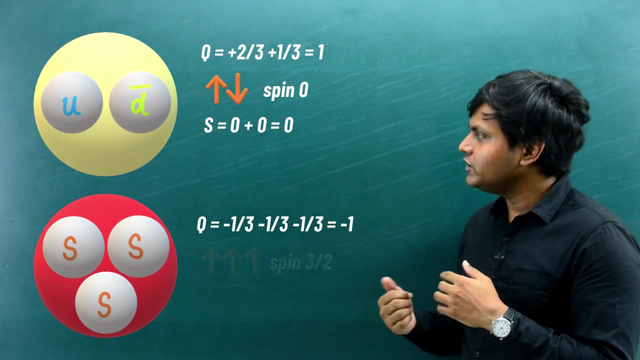 equal to one. So a pi plus has a charge of plus one, while it has a spin of zero and a strangeness of zero, While the omega minus particle has three strange quarks inside them, so it has a charge of minus one by three, minus one by three, minus one by three, which is equal to minus one, while a 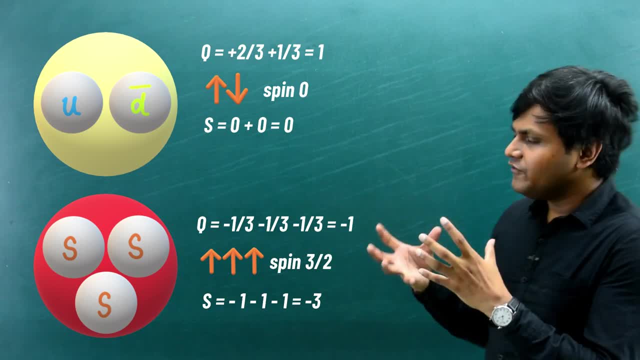 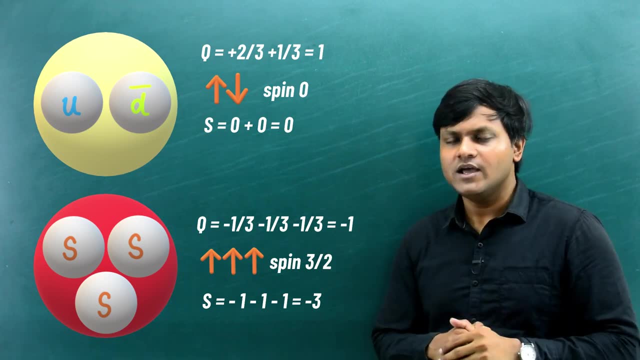 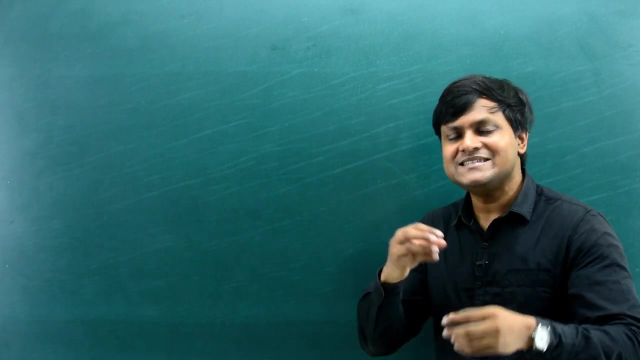 strangeness of minus three. So in this kind of a fashion the quark model can be used to explain the individual properties of all the hadron particles out there. So in a way the eightfold way in particle physics led to the development of quark model, which basically 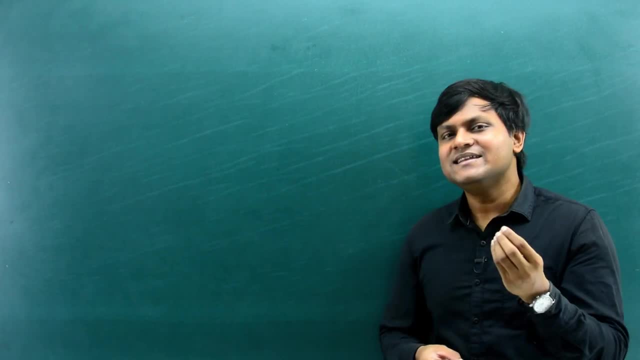 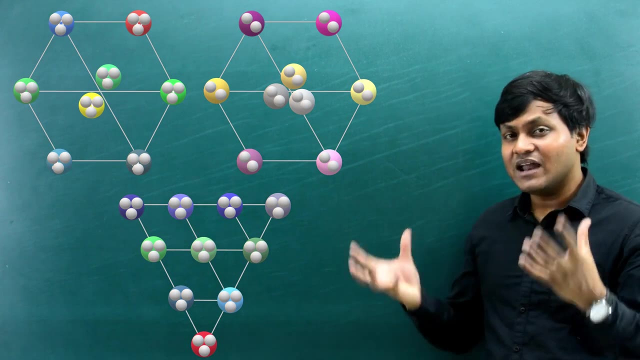 predicted the existence of these fundamental entities called quarks that make up all the hadron particles. So you see how important this kind of a characterization or this kind of a classification was. So this in a way opened up a completely new era in modern physics, because